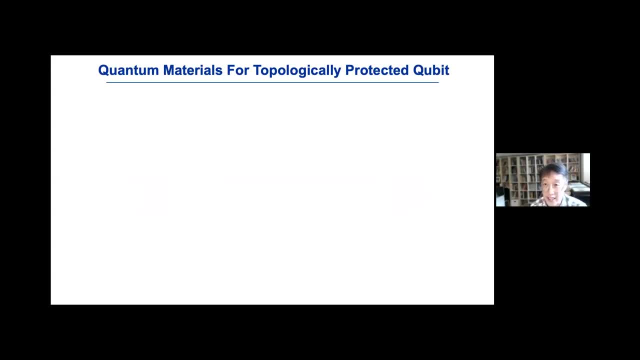 kind of examining through the many different platform one can realize the topologically protected qubits And traditionally this: starting from that, basically by the even denominator fraction of quantum states and using the more real state to realize non-availability, quartz particles into the system, But increasingly that the interest seems to have moved on past the decades. 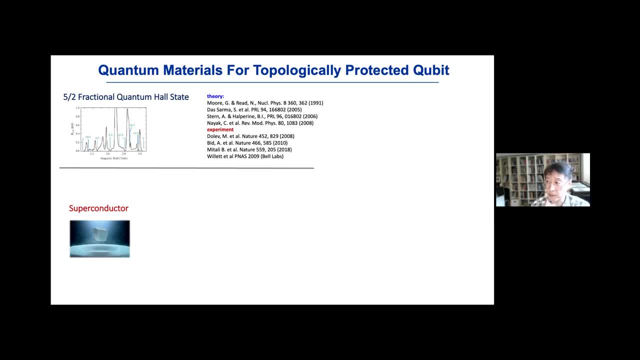 But increasingly that the interest seems to have moved on past the decades. Some sort of combination of the superconductor with the various different material platform, like the topological insulator one, the semiconducting wires or the ferromagnetic atomic chains. 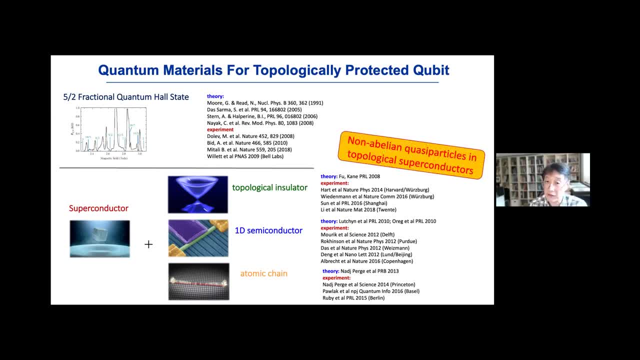 And the goal that the community is setting up is: can we actually realize reliable, non-availability quartz particles and, based on this, topological superconductivity, by proxymatizing some of these topological systems? The why that we've been seeing a lot of the progress, as we heard about. 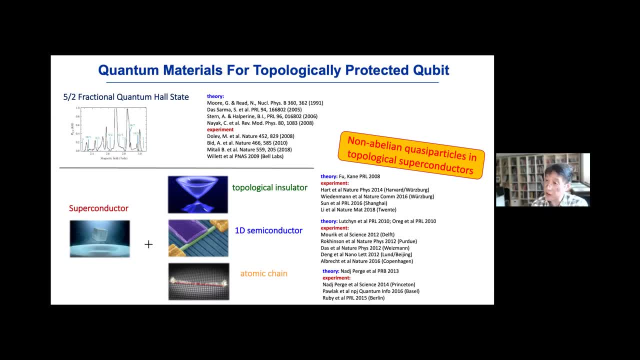 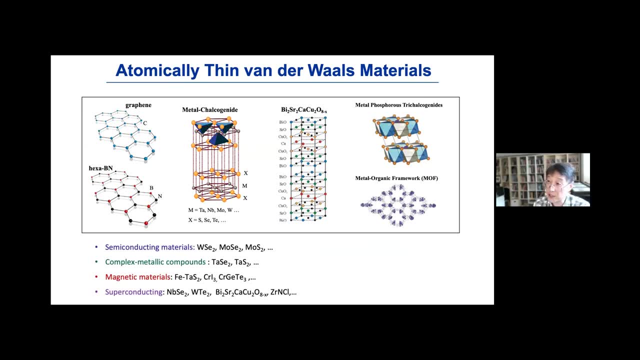 In this workshop. there are yet another material platform. we can also think about moving forward in a similar way, And that's basically this so-called two-dimensional materials or van der Waals materials. We're coming with a many different platform: graphene, boron, nitride, metal, dichalcogenide. 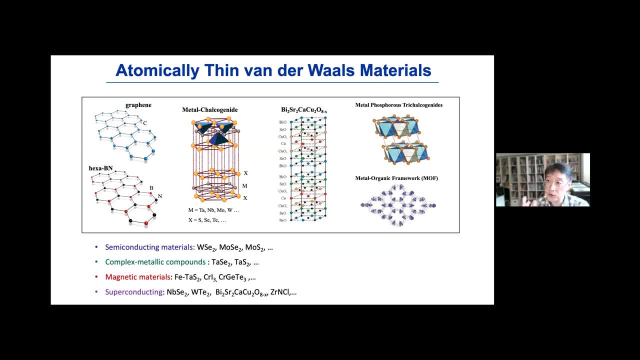 even the cuprate and more of the exotic system. There are many 2D materials available with the various different flavor, including topological insulator Right. Moreover, the possibility of stacking this materials up There is a possibility. we can create some of the functional interfaces that we can rely. 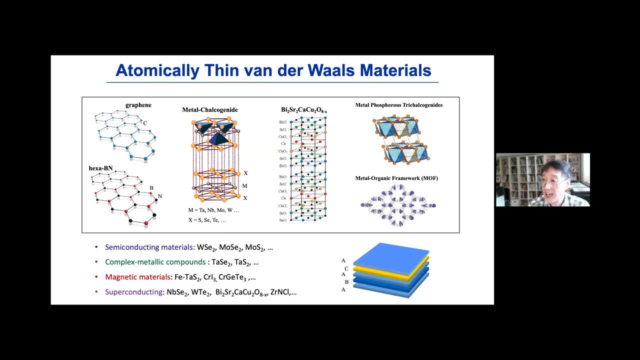 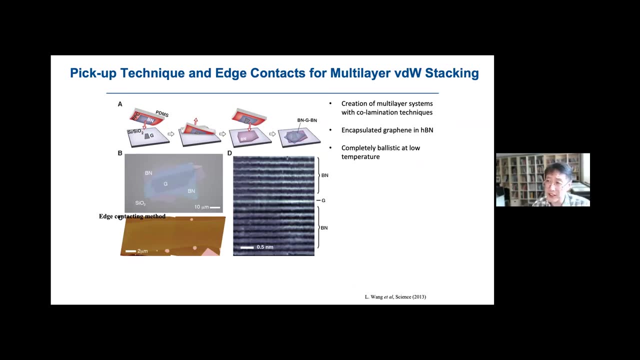 on the as a material platform to realize that the topological superconductivity. Today, what I'm going to just discuss- is just one kind of materials, just the graphene. However, even for the graphene, the recent progress or the community-wise progress, beta- 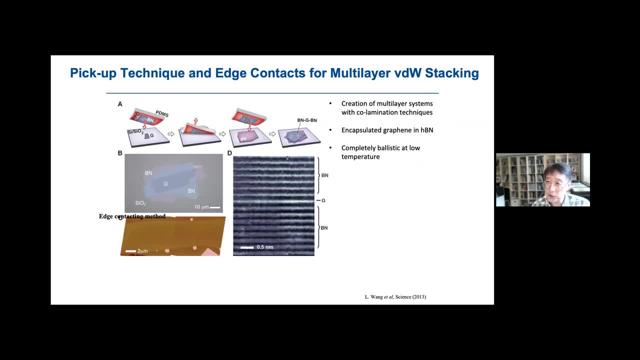 graphene becomes extremely good, high quality 2D materials at this point By combining The boron nitride or all the van der Waals stacks, including all the gates and all the structures. Now the mobility you can achieve in the graphene is extremely high. 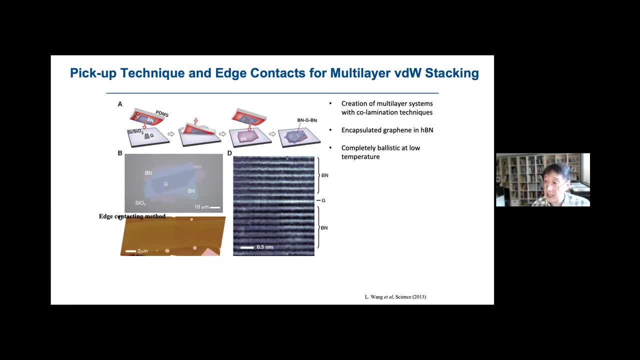 Something like that easily millions or tens of million. It's basically limited by the size of the sample one can get And furthermore, because the graphene is a semi-metal or the zero-gap semiconductor, making contact is reasonably easy. So making the various contact, including the superconducting contact, 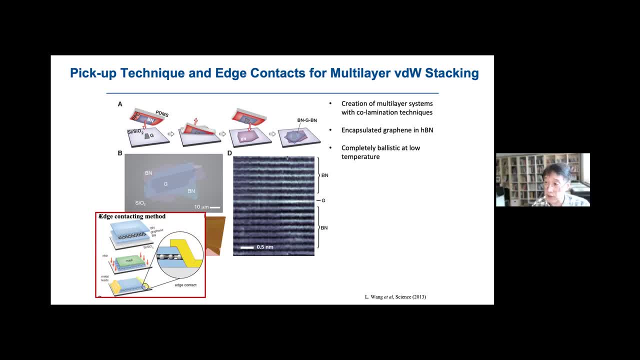 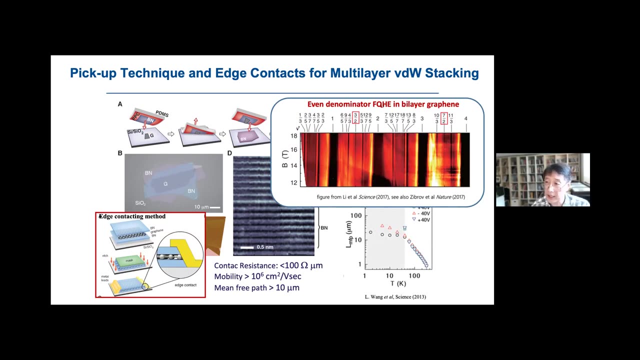 Is a reasonably easier than a semi-conducting platform, And this will immediately give us some of the advantage to using the graphene as a one interesting platform. And quite recently I think it's been demonstrated- This is a result from the Corey Dean's group at the Cornell, the Columbia, demonstrating 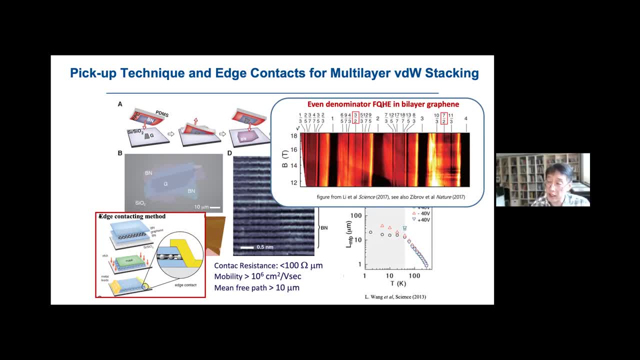 that we didn't, the lab chip, magnetic field. They can demonstrate the all the subtraction of quantum or effect down to even denominator states in the realizing the bi-layer graphene. And this is basically, And this basically give us some hope that maybe we can just use the graphene as a material. 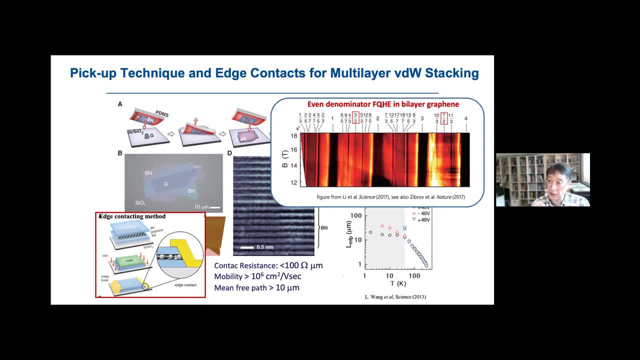 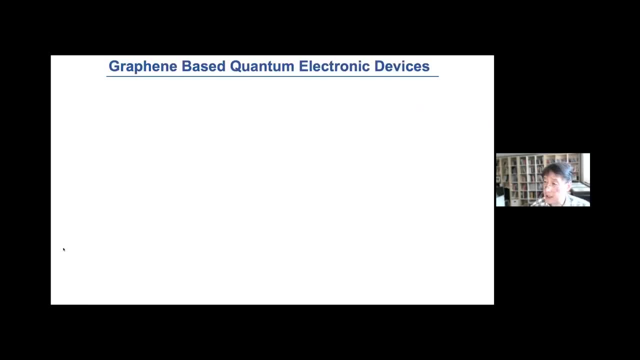 platform to combine with the some things that the getting into the district creating topologically protected Now, and the other. the other part is that the a lot of the the gates and the contact control is also possible Now. the state of the graphene fabrications now allows us to make the graphene rather 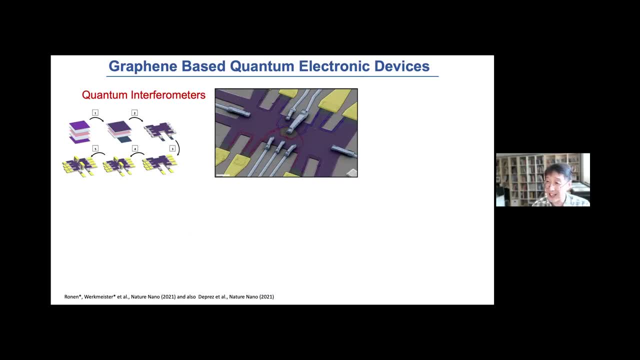 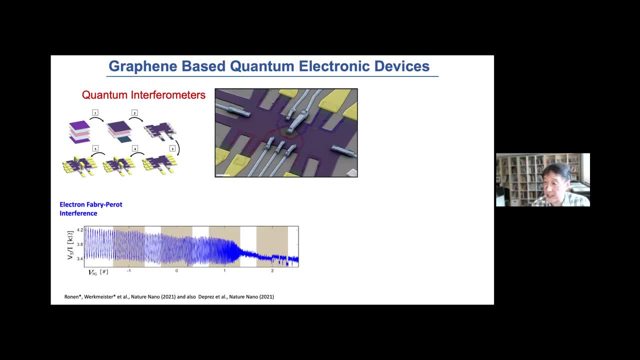 A list of. we started getting this interference in the integers and pushing it to the distractions and hopefully bring it to the more of this, the even the name you're in a mineral states and bring this graphic as an important material platform or so realizing this quantum or based on the topological curates. 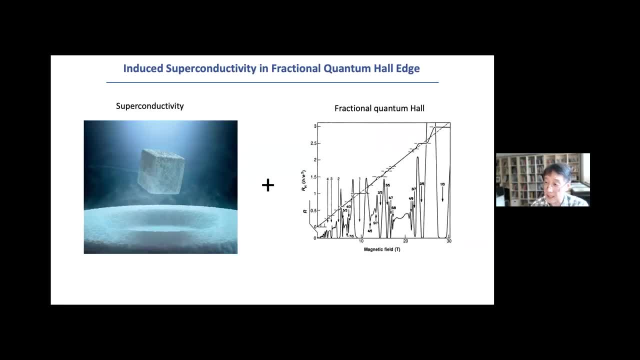 Now, today I'm not going to dwell on this one but particular topic I'm going to discuss today is basically using the graphic as a material platform to realize combining the superconductivity and fractional quantum effect. try to bring this as the first step toward the topologically protected qubits Right, The idea about combining the 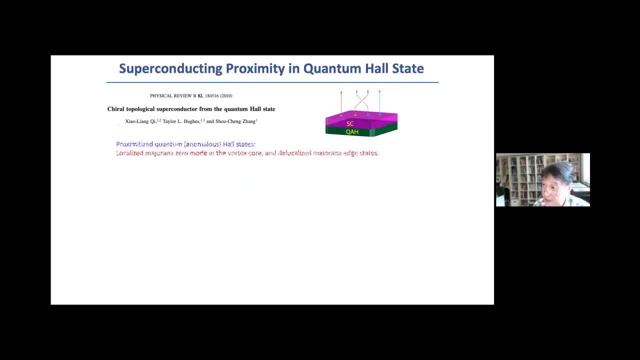 superconductivity and quantum effect has been around. One of these first ideas came around the Xu Cheng Zhang's work that basically proposed that, combining superconductor with the quantum Hall effect or quantum onomalous Hall effect, one can create this topological superconductivity. 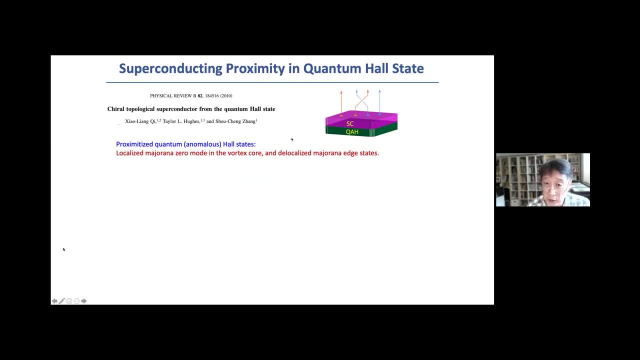 proximitize the topological superconductivity, for example, and the vortices on this type of the combined system should contain the Majorana zero mode in there and manipulating that one can just realize some of the topological superconductivity with the Majorana zero mode. that. 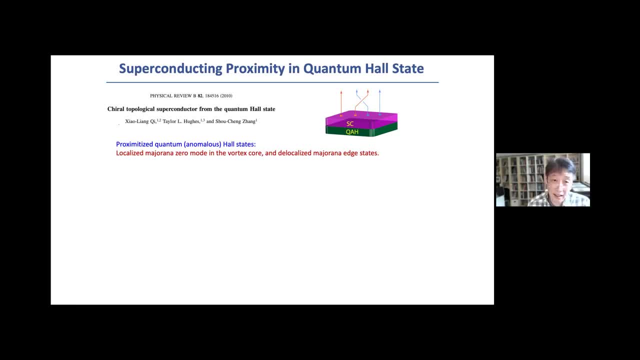 nucleate the defects. In fact, this idea that around the first, proposed in 2010, quickly just pushed that even forward. What if now, instead of the combining superconductor with the integer quantum Hall effect, what if we just combine that superconductor with the fractional quantum? 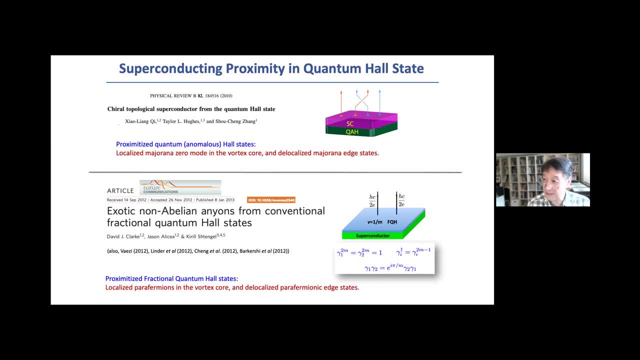 Hall effect Within a few years. there are several groups, many of the authors in fact, in these conferences collectively come up with the idea that indeed, if you combine that superconductivity with the fractional quantum Hall effect, you can realize it, generalize. 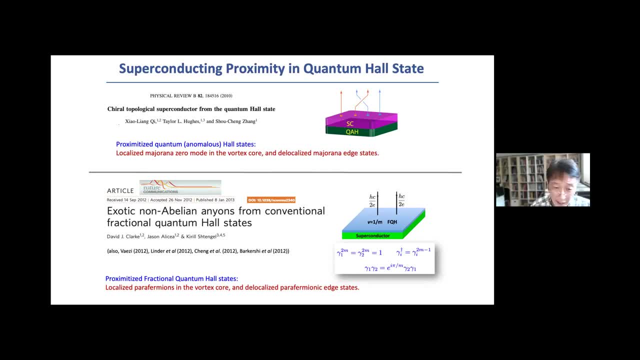 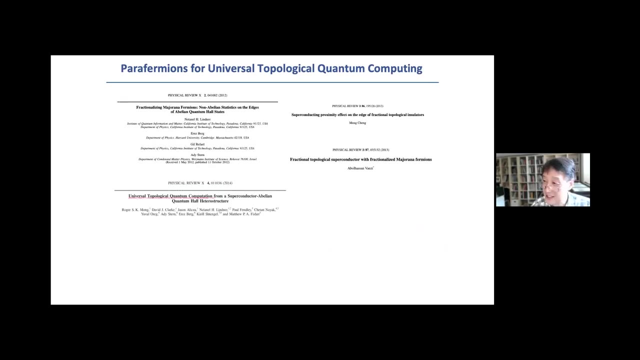 the Majorana mode or the nanovillain anions called the parafermions, with the multiple grounds, Data is possible, right, So it is in some sense to generalize my minor on the board And this parafermions platform. if they do exist, it can be used as just the more close to universal. 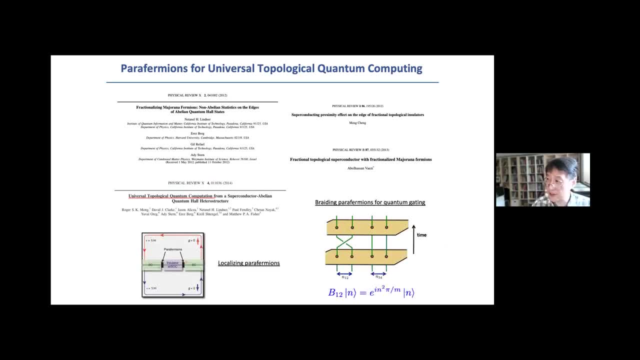 quantum computations. I think that's kind of one of the real excitement that maybe just pushing this idea to combining the superconductivity with the fractional quantum Hall effect, One can go even further beyond this. They might on the physics that we are looking for. 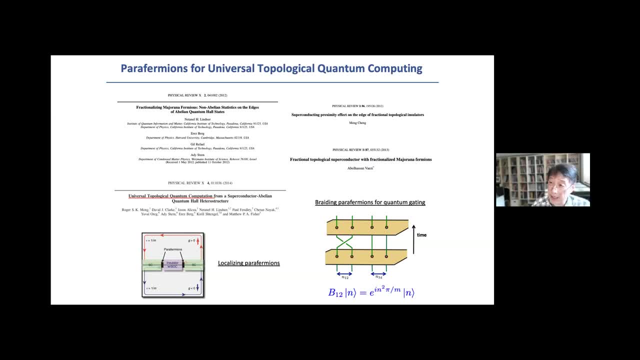 While the theory proposal is out there also the idea of the combining the superconductor with the quantum Hall system has been around almost two or three decades- quite a long time- And in particular that tries to combine with the superconductivity of fractional quantum. 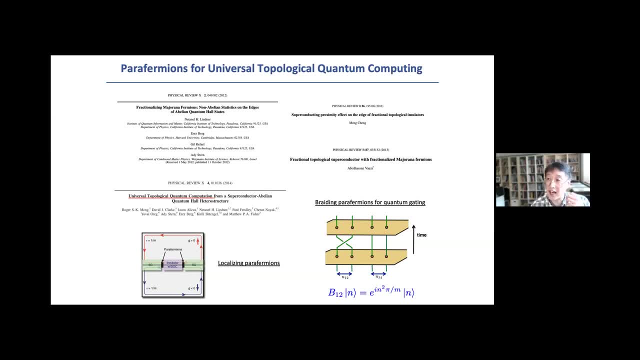 Hall effect. you need to come up with the idea that how to make good contact with the superconductor which actually has a very high IC2, such that the superconductivity can survive with a reasonable magnetic field that one can set up to realize the fractional quantum Hall effect. 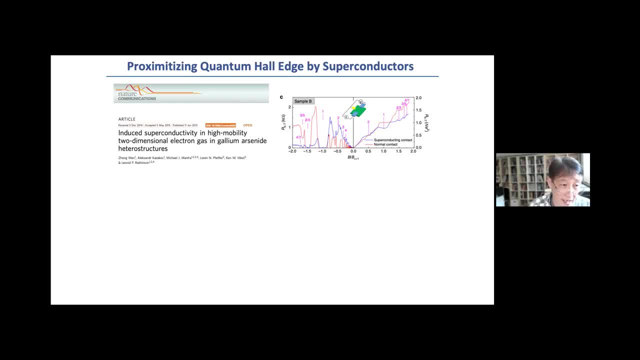 One of the notable example is here. It was done by the Leonie Rockins at Purdue in 2014.. They just used the gallium arsenide, the two that combining with the Niobium superconductor, where the fractional quantum Hall effect sets in the few Tesla, which is well below that HEC2 of 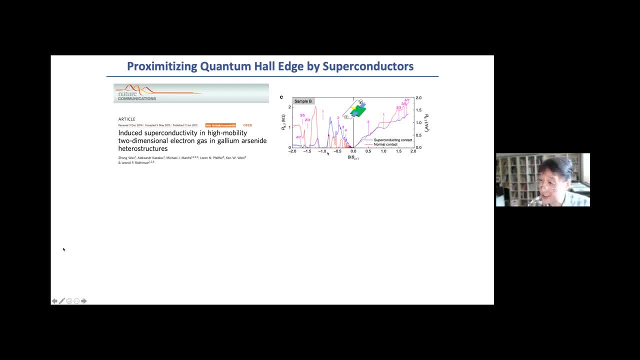 the Niobium, And they demonstrate at least that they can use the superconducting contact to measure this fractional quantum Hall effect. While this gives us an intriguing result, as you're showing here, making this reliable contact with the Niobium, with this semiconductor, was not too easy. Part of the reason is well. 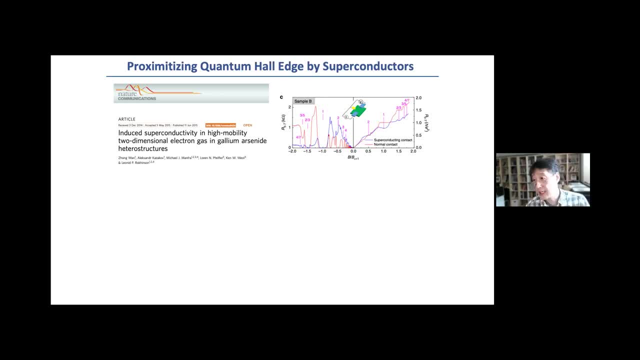 that you have to really fight with the short-term barriers, especially coming from this refractory metal like the Niobium, And that's been kind of struggle and making reliable contact with the semiconducting the material has been some of the big technical challenges, Of course there, as I said, 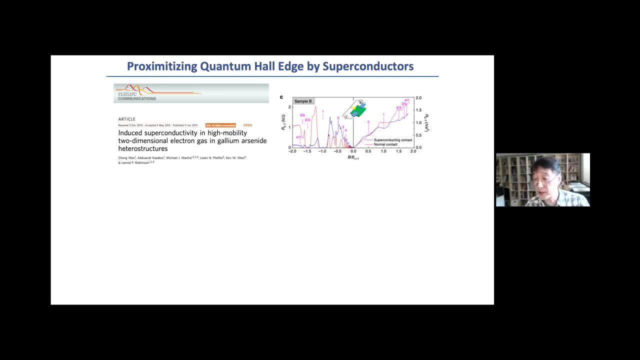 graphene has an advantage because there's no gap in principle, the semiconductor gap. So therefore you can make this a decent contact with many different material, including the Niobium or the Molybdenum And those kinds of type two material with reasonably high. 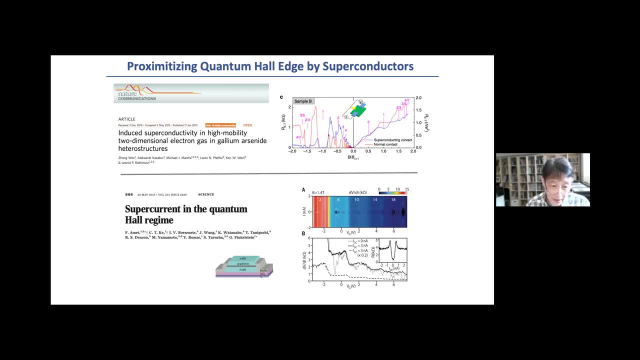 HEC2.. And here's another example, the one example that Gladden-Kunzstein's group actually demonstrated, with many other groups as a similar result: making the good contact with, in this particular case, molybdenum, with graphene as a channel. 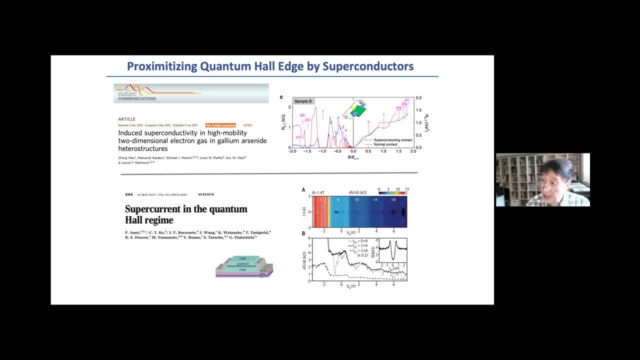 and they apply the magnetic field, the graphene get into the quantum mole region and then yet the superconductivity in the molybdenum is survived. So in this particular example they demonstrated that coexistence of the quantum mole appears a plateau in the two terminal conductance. 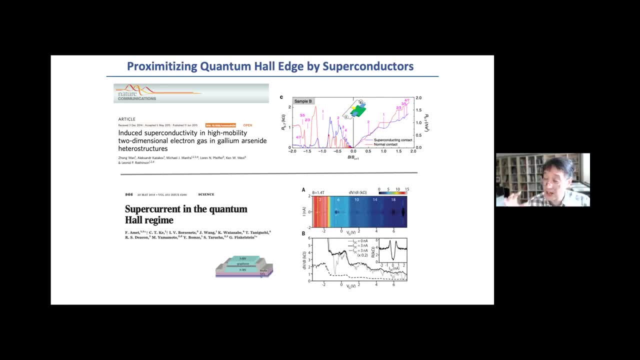 At the same time they demonstrated that there is a Josephson effect appears between these two superconductor through this quantum mole channels in between. However, this is not precisely coexistence in a sense. by definition. having Josephson effect means you need kind of zero resistance. 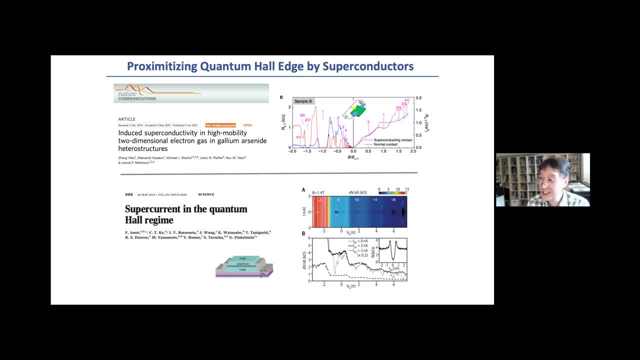 In quantum mole in two terminal you have always kind of quantum mole plateau. So what they see is in the middle of the quantum mole plateau. sometimes it's the resistance dip into zero to show the Josephson effect in the middle of the plateau. 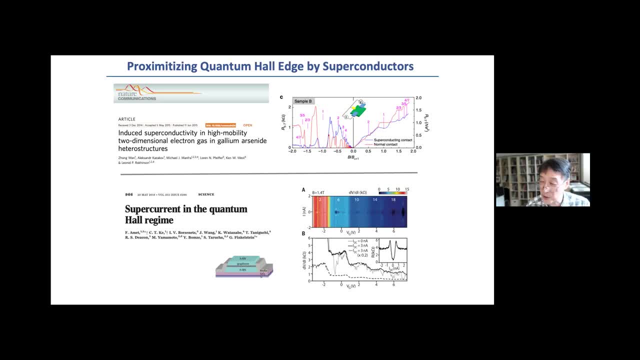 So there is a alternation of the quantum mole physics and the Josephson effect in there, but it's not necessarily kind of truly coexistence cases in this particular case. But this bring us some of the interesting questions we can just look for Instead of using the Josephson effect. 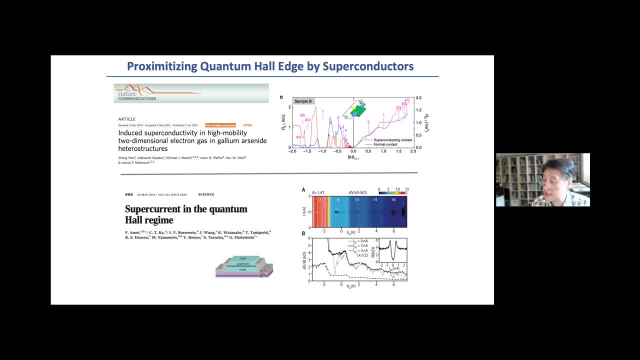 can we actually just really probe that coexistence between superconductivity or proximitized quantum or edges together with the? the prove the coexistence, superconductivity and quantum mole physics by just showing the proximitized quantum or edges. One of the idea here is using Paphos-Josephson junction. 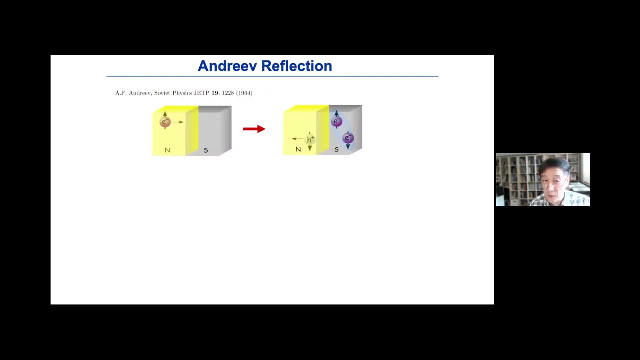 In other words, just kind of use Andreev reflections. Well, we know that in Andreev reflections and when carriers coming from the normal metal to the superconducting interface you can inject the Cooper pair into the superconductors by having this at the retro. 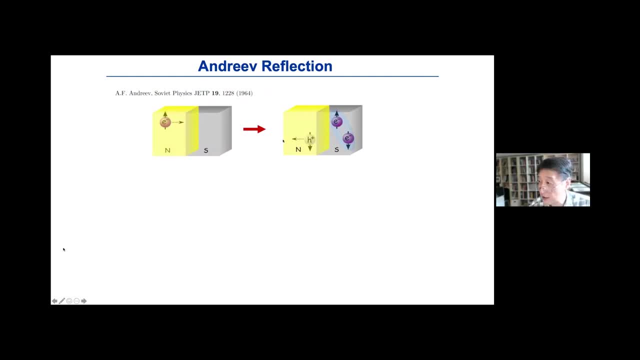 retro the holes back from the interfaces, right? So idea is, instead of using the normal metal, can I just deliver the current through the, the quantum or edges state, to the superconductor and just can detect this, the holes coming off from this Andreev reflection process. 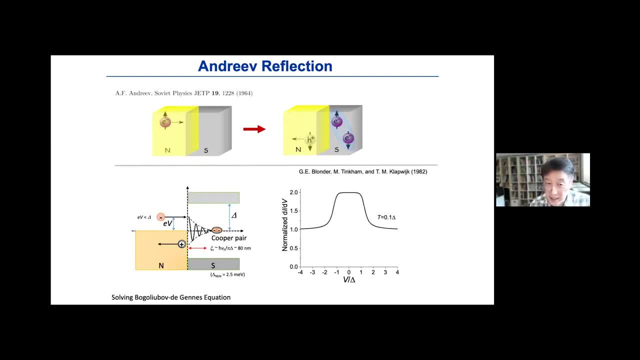 The this Andreev reflections usually appears as an enhancement of the interfacial conductance and the zero magnetic field. basically, just looking at the how the conductance got enhanced will tells us that how perfect is the interface between the superconductor and the normal metal. 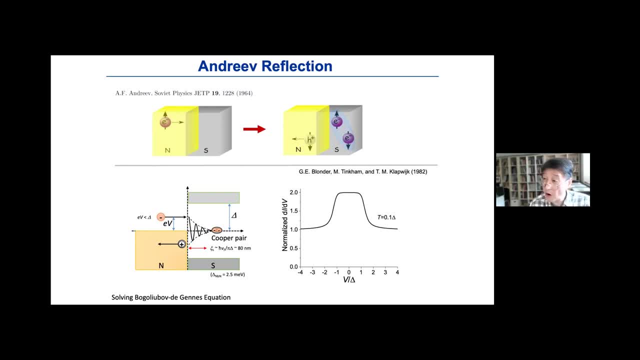 And this enhancement can go up to the a hundred percent, because all the electron gets in reflect by the hole. Basically I have a hundred percent Andreev reflections And then I expect to see the a hundred percent enhancement. Of course the interface is not perfect. 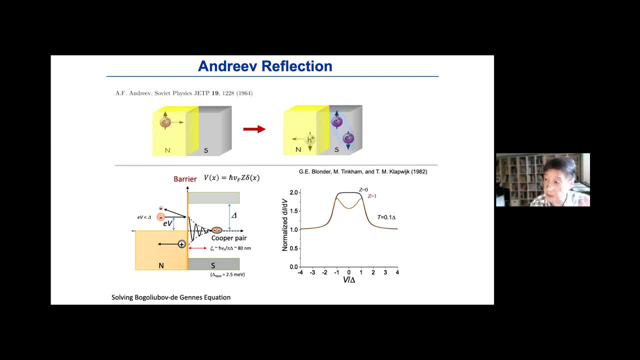 And you started kind of develop some barriers and whatever barrier it is. And then if the Andreev process start to reduce, then of course conductance enhancement to reduce Eventually. if this is completed, tunneling of the free carriers- then you expect to see that this tunneling conductance. 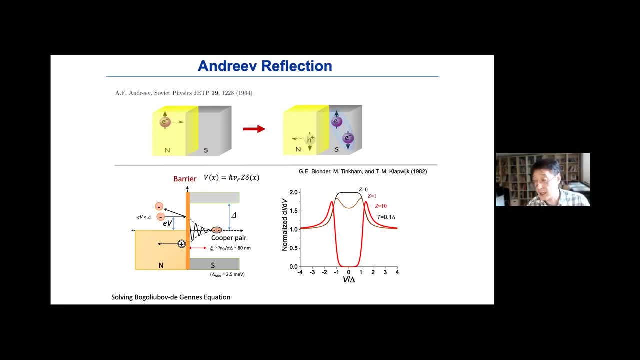 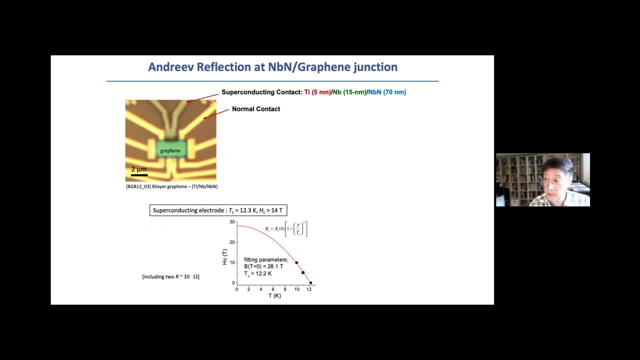 type of the measurement was complete suppression of the conductors in between. So idea is the first: can we actually build up the soup conductor and the graphing channel and demonstrated whether enough the under reflection can be measured under the presence of the magnetic field? 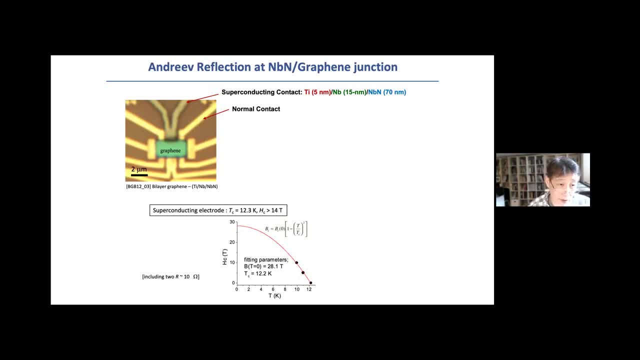 So here's an example that here that we use a graphing and then as the soup conductor, we particularly use this, the combination of a Nivium and Nivium nitride. use titanium as sticking layer And this the combination provide us. 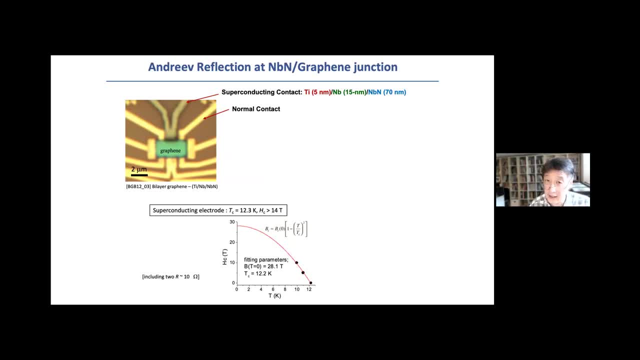 extremely efficient contact to the graphing through the tie layer, but presence of the big presence of the Nivium nitride give us a quite high HEC2.. In fact, our estimation of HEC2 in this device is a way beyond the 20 Tesla. somewhere in the 25 Tesla to 30 Tesla. This is high enough magnetic field that one can, in principle, realize the fully developed diffraction of quantum or affecting the graphing channel, with a decent graphing devices. Indeed, when we measure the under reflection, 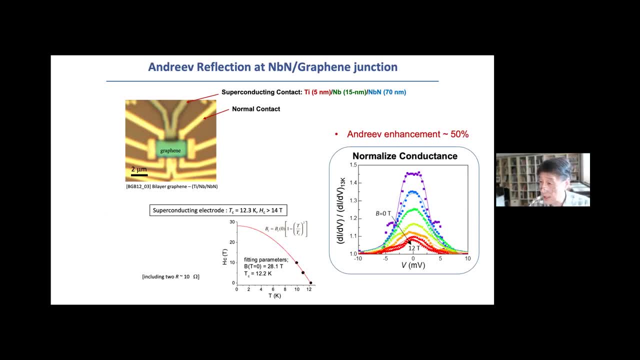 in this type of device with this combination we see that in the zero magnetic field, about the 50% of this, the conductance enhancement, indicating that indeed we can make the fairly good contact onto this device And with the magnetic field, of course. 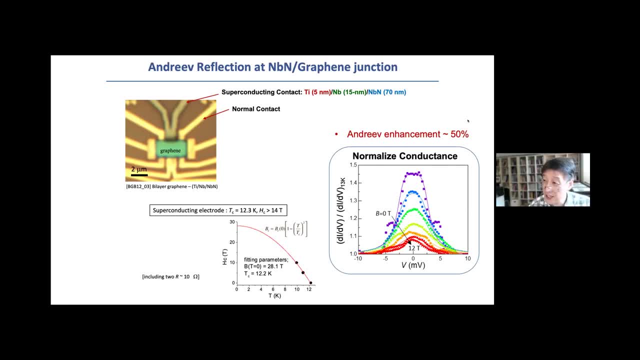 with various regions, the vortex formations or various regions, this conductance enhancement actually reduced. in other words, the unreflections efficiency reduced plus the up to the 20, 12 Tesla, you get about 10% of enhancement. So it's- I think it's still reasonably effective. 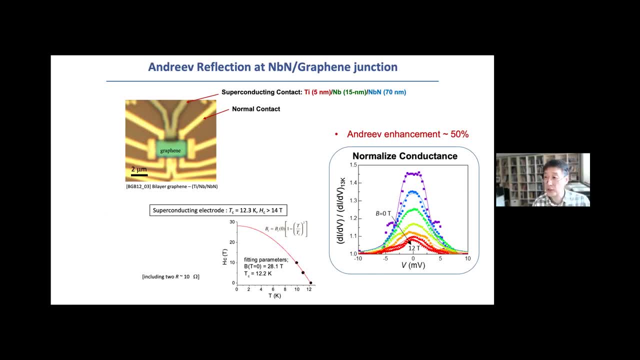 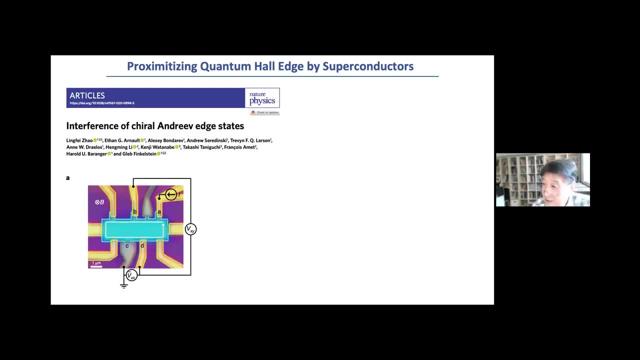 such that we can realize the experiments that by combining that quantum or edges with the superconductor, So what you can observe. so very similar device. but I'm just using again Gloucester and Kirstein's recent experiments to showing that how the under reflections work. 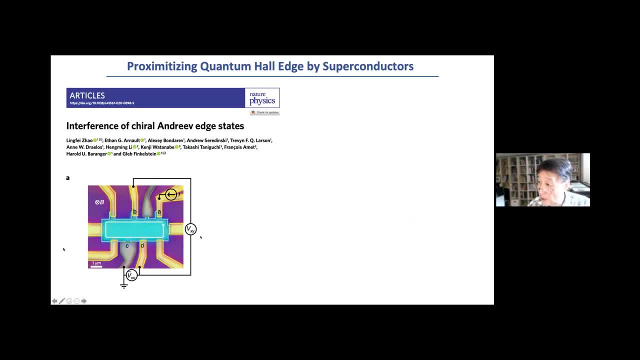 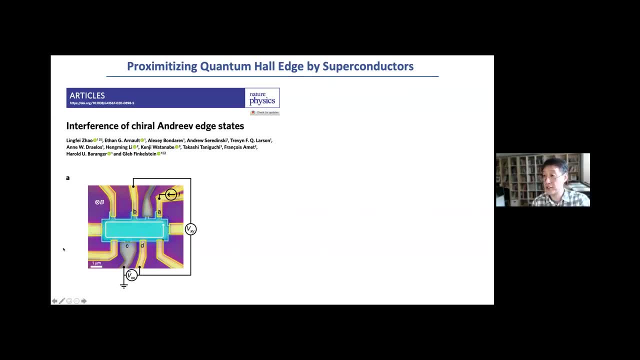 down flow of the quantum or edges state, chemical potentials. So now, what do you expect to see? that is, when the electrons bump on the superconductor, it will just kind of go through this under process, each under reflection process, convert electron to the hole. 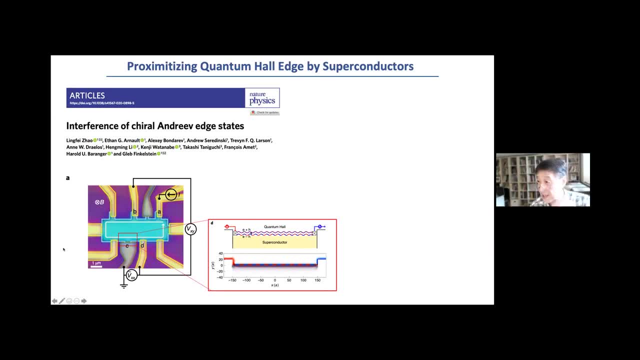 And again whole downstream hole we processed in the same direction and that hole will just convert into the electrons and holes and that right. So you can see that there is a successive through a transform, the electron and holes, when this quantum energy states are just traveling. 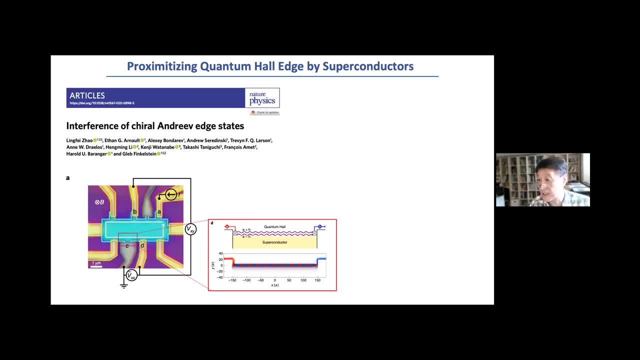 across the superconductor, where you keep just getting into the superconductor to create this group of pairs, right, And this process. eventually, if the superconductor is long enough, then we'll mix up the electron holes And then in the downstream, 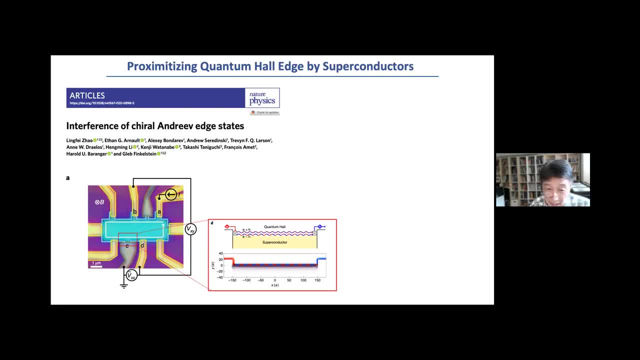 basically some of the mixture between the electron hole and detail depends on the length and then all the kind of geometries and scattering process of these cases. So, but in the end of the day, in the downstream of the quantum orages, you will see that it's just basically mixtures. 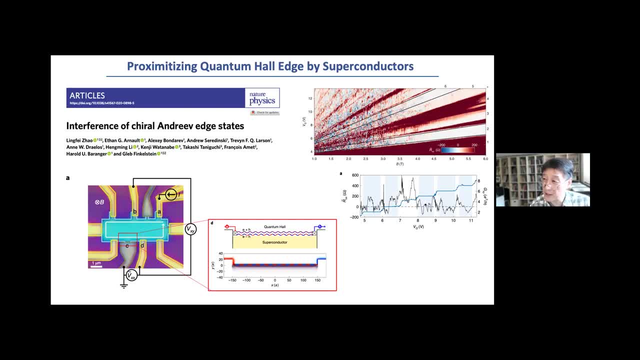 of the electrons hole, which actually can sensibly tune by the gate voltage and magnetic field. Indeed, what the Finkelstein group actually observe is, if you just carefully monitor the downstream, the quantum or the chemical potentials, you'll see that there's a lot of defined fluctuations. 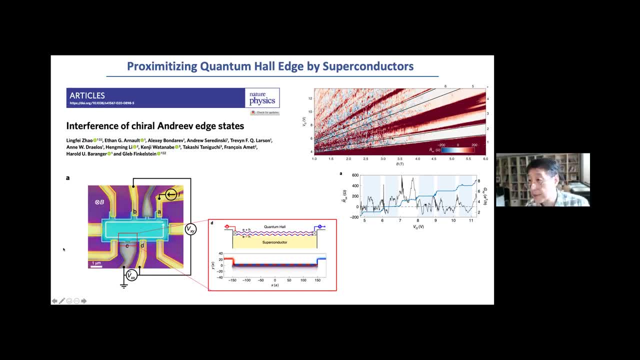 of the chemical potential of the downstream of the quantum orages more like the symmetric C-shape from the zero the positive and negative is rapidly processing. Part of the reason is basically, as you change the gate voltage or magnetic field, that, whether final electrons comes out. 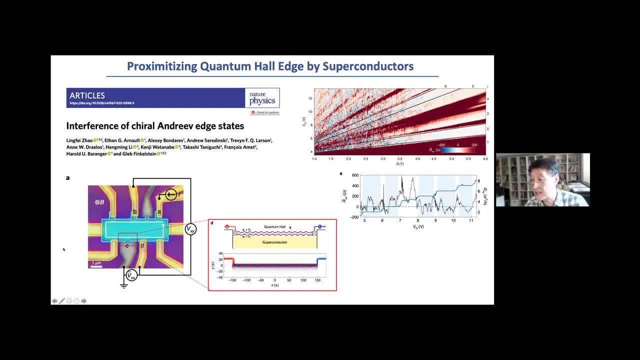 hole comes out depends on the details of the system, right? So why do you see that there is the Andreev-Egyt process, or Andreev states? the Egyt state forms along the superconductor. This may not be too useful for now, right? 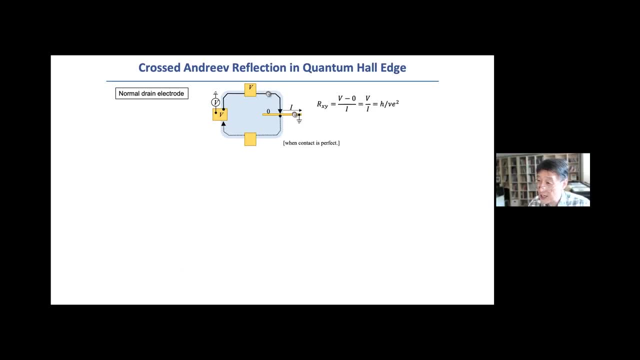 Although there's an interesting effect we can see as fluctuations. However, this actually give us kind of another idea. Maybe we can proceed a slightly different way and give it some differences. So imagine that I have this quantum or states, quantum or the samples. 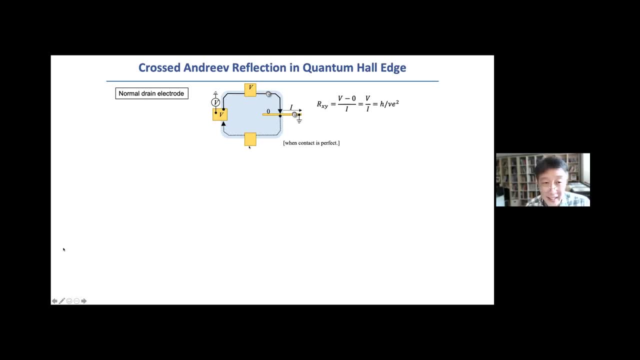 and with the four normal contact is the connected. So typical way that I can measure this multi-terminal measurement is I just bias or the one of the contact and ground one of the contact and measure the voltage in the upstream and downstream and basically this upstream voltage. 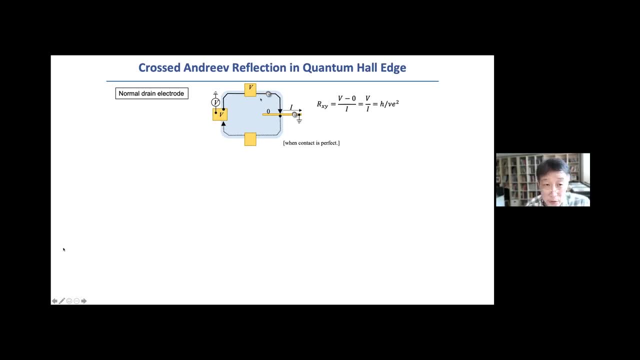 and downstream voltage. by the way, this is a should be zero right And I will get this whole resistance Rxy by just reading off this two voltage difference and divide by the current right. So that's kind of typical quantum or physics. 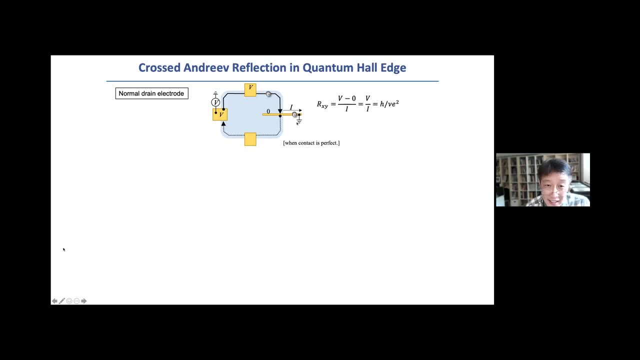 What if now I just replace this contact, especially this ground contact, with the superconductor? Now, when I just replace with superconductor, as I just briefly explained, when electron comes in, electron will be placed to the hole and electron hole 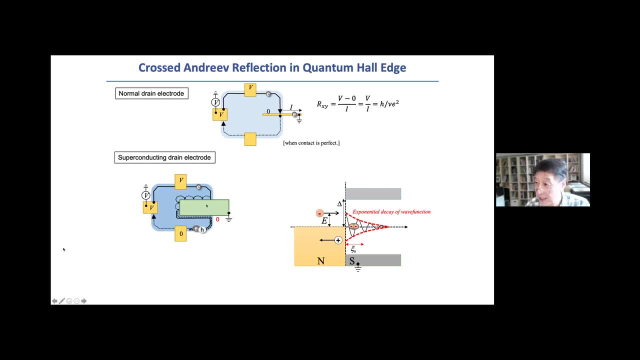 and you start to see that this andriva state is happening. As I mentioned, if the discount, the superconductor, is this length of the contact is long, eventually you will just mixed up all the electron holes in downstream. you get more like the mixtures right. 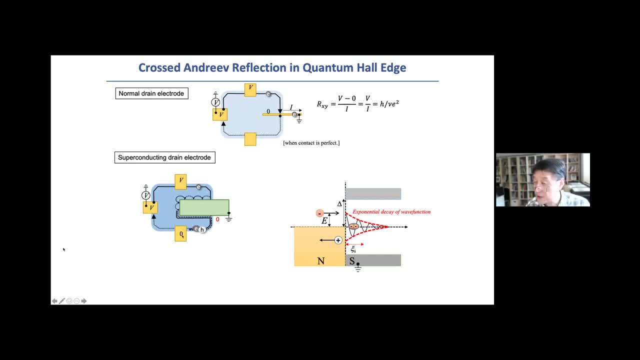 Although they are fluctuating. but if you just average over more of the you get the zero. So as if that, if I just measured the whole voltages, nothing changes. suppose changes when the system get into, when system get it. 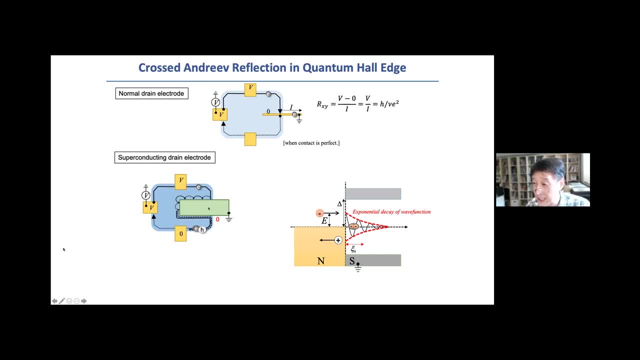 when this contact is replaced by the superconductor right And the, every times that this, the andriva process is happening, then when you have this, the electron group of pair, whole group of pairs, that getting into the, this superconductors right. 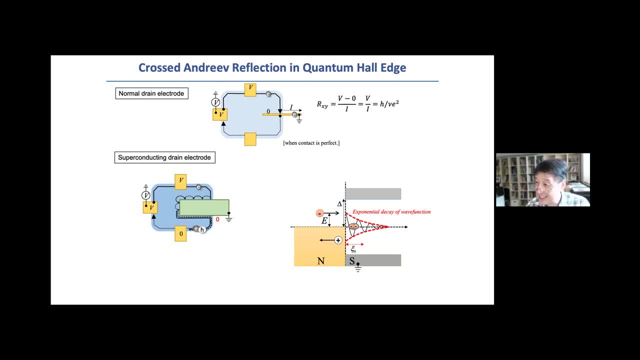 What if? now, though, if I just make that this superconductor thin, such that, across this superconductor, basically, that the instead of the- you get this- the group of pair forms by just combining this andriva process in one side? 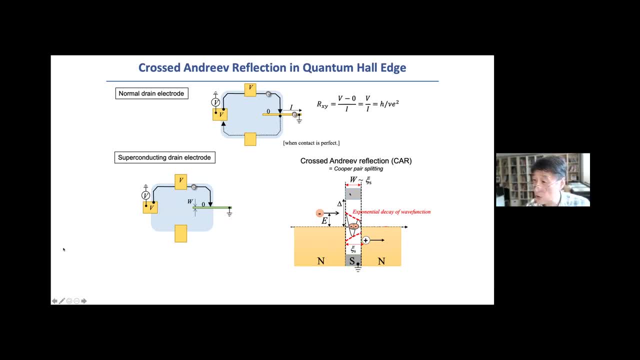 what if that superconductor itself is thin enough to compare with the superconductor quadrants length, such that whole is not graphed from the same side of the contact, but whole can be graphed from the other side of the contact, And this is what you call the cross andriva reflection. 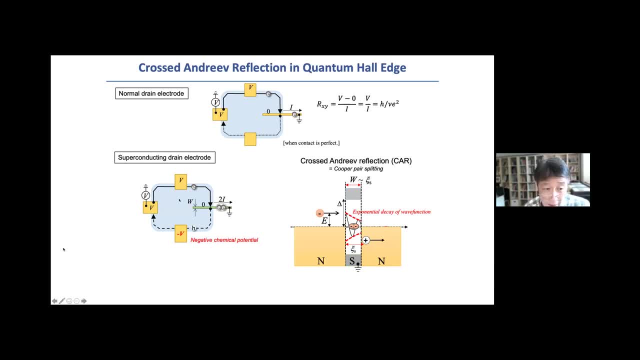 If that is happening and if that is dominant process, what we expect to see is the electron comes in, will directly convert to the whole And I expect to see in the only in the downstream- just to read the downstream negative whole voltages on. 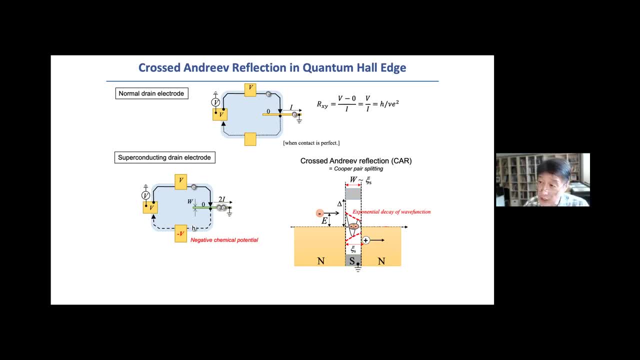 Right, And so basically that's the idea that instead of fluctuation, I should be able to see the solid and negative signal in the downstream of the, this quantum orages. So that's basically idea that we are going to use, and just use this cross andriva reflections. 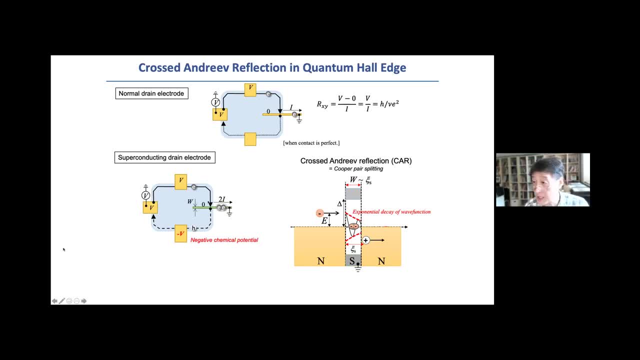 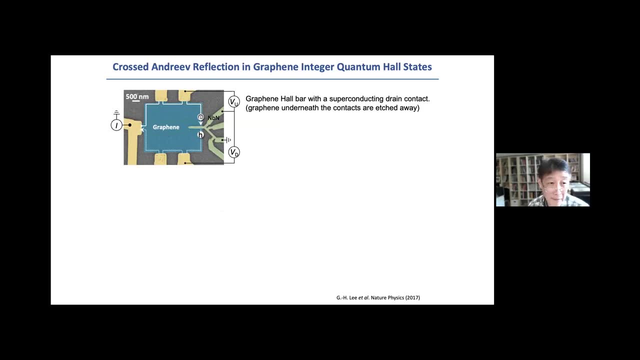 We want to kind of show that, indeed, this quantum orages, incoming quantum orages, are the proximate ties by the superconductors, right Indeed, this experiment actually worked it out a few years ago already. Here, that is a graphene and nitrogen nitride electrode. 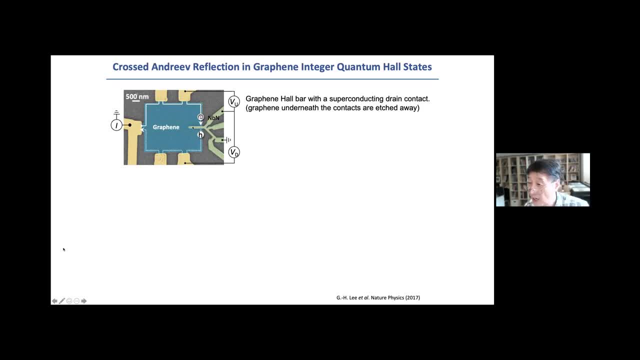 except now the nitrogen nitride electrode is so thin, something like the order of a hundred nanometers or even less. right And measuring the sand at the bias, the upper side of the quantum orages and ground with the superconductor. 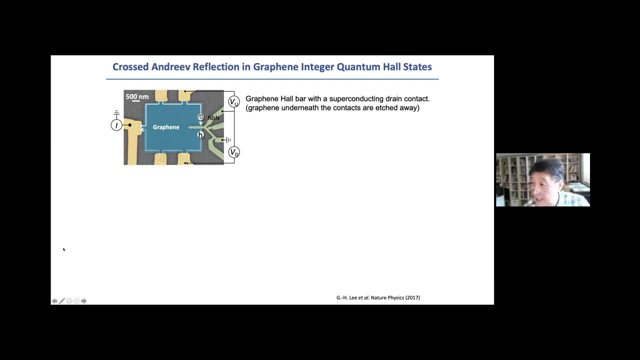 And we monitor the downstream of the chemical potentials and that normalize the chemical potential with the current And that is what you call the cross andriva reflections, resistance, And then, indeed, whenever, when we see that the quantum or is a well-developed 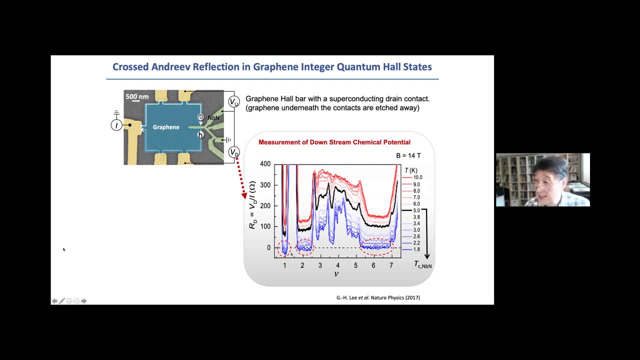 like the six, two and one single layer, the quantum or effects in graphene. we do see that indeed the downstream of this chemical potential is deep into the negative side. You see that signal is not necessarily big something, even in the nuclear one. 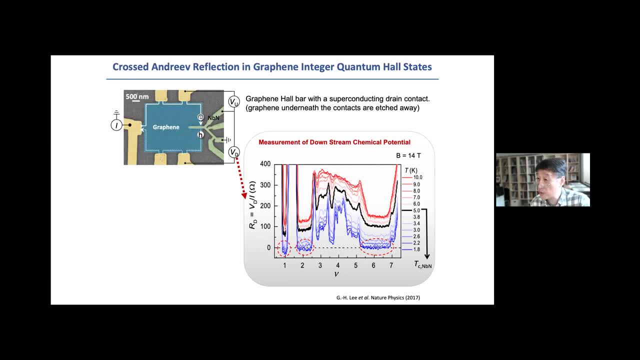 we get about 50 ohmish of the resistance, of the resistance Which we supposed to get, about 25 kilohm. It's a very small, it's about few percent, about 1% or few percent of the signal. 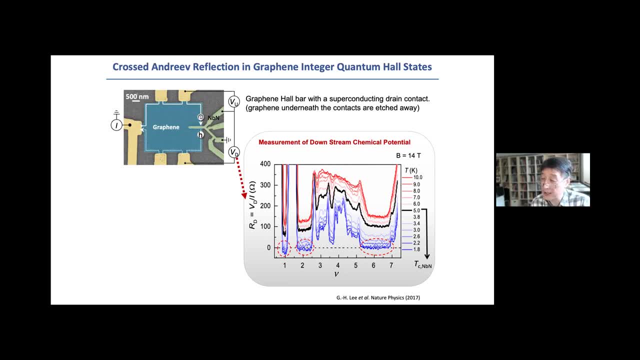 but clearly that negative signal is well beyond that. There were detection limits indicating that indeed we can make that this the cross andriva reflection across this superconductor. Now, one of the idea that just viewing this cross andriva reflection is using the concepts of the 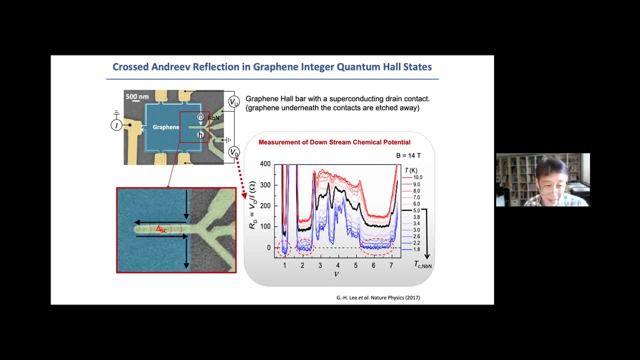 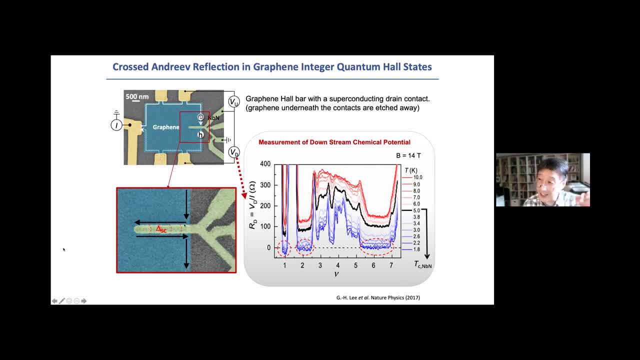 Now the? when we make that, the contact, we basically remove the graphene underneath and backfill with this superconductor, right? So for a moment, if there's no superconductor, basically quantum or edge state, we'll just follow through the French. 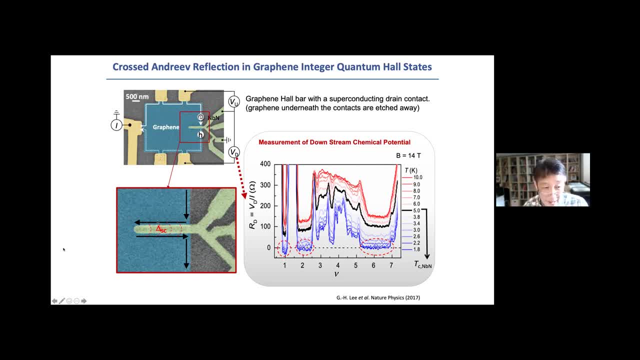 we created like this. Now, presence of superconductor is basically the coupling. This two counter propagate in terms of spatial direction of the quantum or edges through the superconductor. Basically this has a very similar flavor. can create this the Majorana AG state. 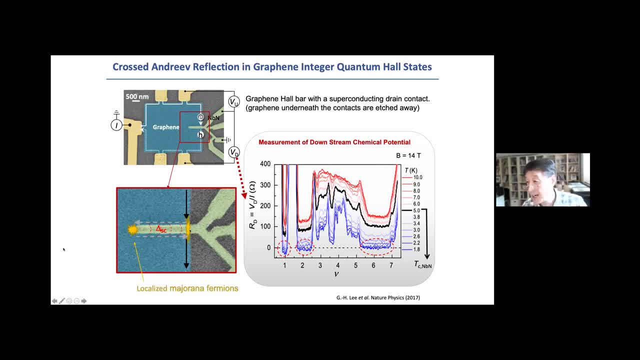 Majorana state zero mode onto the, this quantum, the semiconducting wires in very similar formats. So one can just view this type of this cross, unduly reflections combined with a very thin superconducting contact. as an analog of this, the forming Majorana zero mode and semiconducting nanowires. 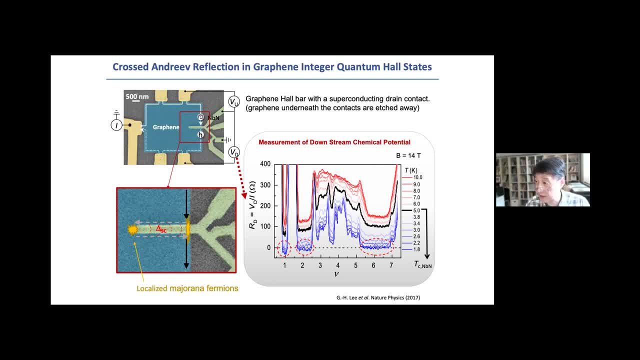 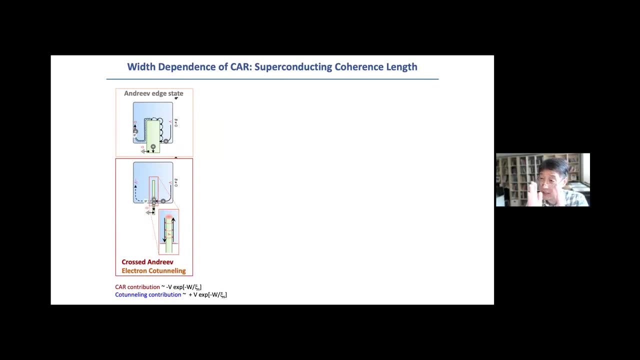 with the superconducting super, the proximate superconductivities, right? How do I know that this is really the case? One way you can test that out is basically varying this width of the superconductor. right, Because we know that the superconductor need to be thinner. 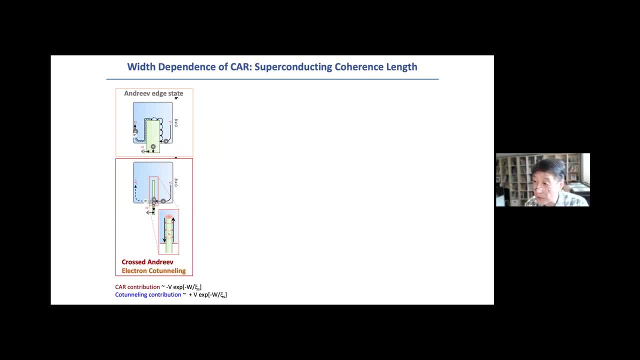 than the superconducting coherence length to provide the cross unduly reflections. If indeed we make the superconductor thicker and thicker, we expect to see that the signal will quickly go away. Indeed, if we just varying this superconducting wire, 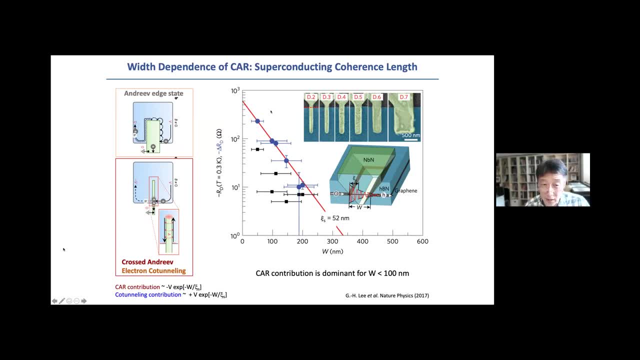 the contact, the width from, say, 100 nanometer below 100 nanometer. through this, something with a few hundred nanometer, you can see that those kinds of the negative signal we are getting exponentially decays with this width of the superconductor. 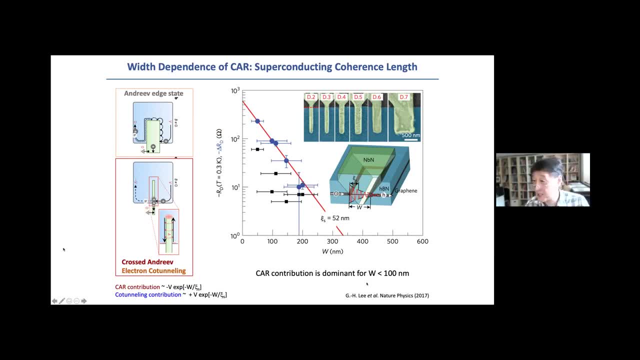 And that the parameter we can extract out of this is basically the superconducting coherence length, which is about kind of 50 nanometer-ish of the length scale which more or less agrees with what we expect to see that in a nirum nitride, the superconductor 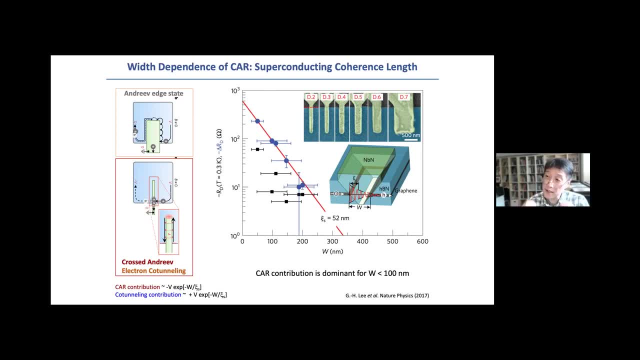 So at least we know that the basic idea of using this cross unduly reflections to just probe the proximate, proximate ties of quantum energy seems to work. Now the next level here is: can we actually just push this into the now? 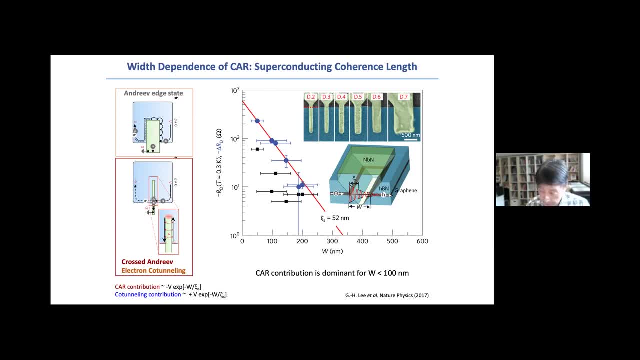 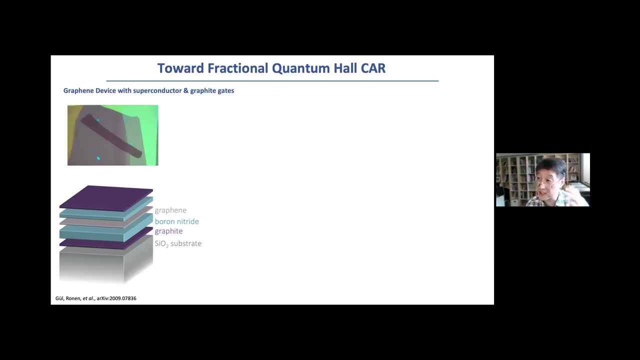 not only integer quantum all, but fractional quantum all in fact. For there we need kind of the just bring up, boost up the our device verification even further. What we need is an extremely high quality graphing channel to realize this type of experiments. 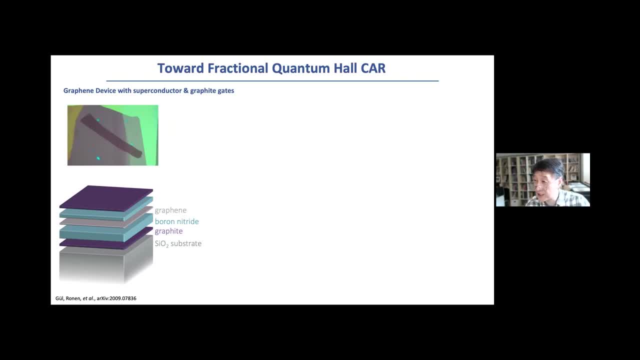 So we have to bring up this, the graphing encapsulated bottom nitride, and, more critically, that we have to put this top and bottom graphite gate, provide completely bandwidth stacks and without any impurities, and then fabricate the devices out of it. 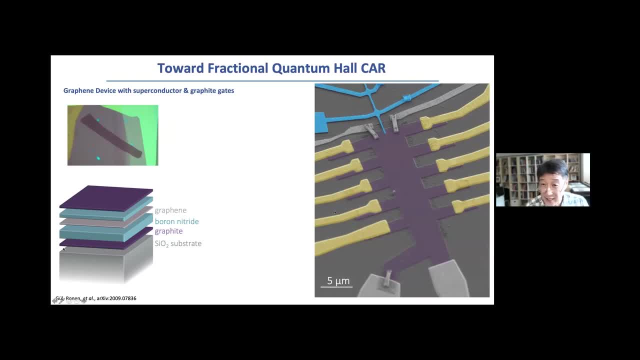 It's challenging, it's doable. Here's the device, the overall images. And this is normal. the gold color is a normal contact made of the tie gold And here is basically this the science. the advanced rotation color is the narrow nitrogen-nitride contact. especially essential part is end of the 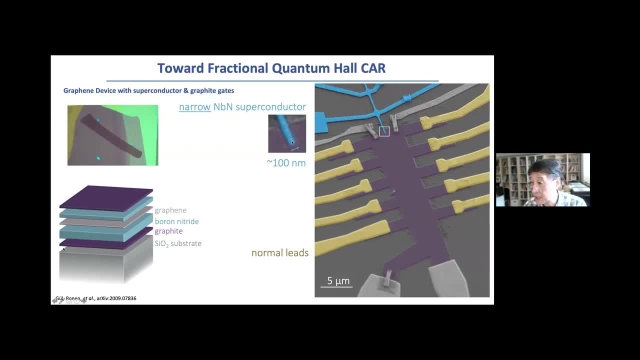 this nitrogen-nitride contact Width is about 100 nanometer, even less right, And then the, as I said, that graphene underneath of this contact is removed first and backfilled with the nitrogen-nitride. So you can think about this: is a trench of the graphene channels, backfilled. 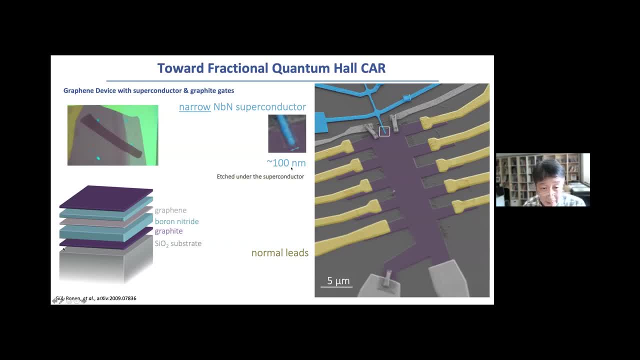 with this superconductor. And another important aspect is we have to carefully actually weight this top graphite, the gate, such that in fact, that there is a region of this, the around this superconductor region, where we can separately control this density. 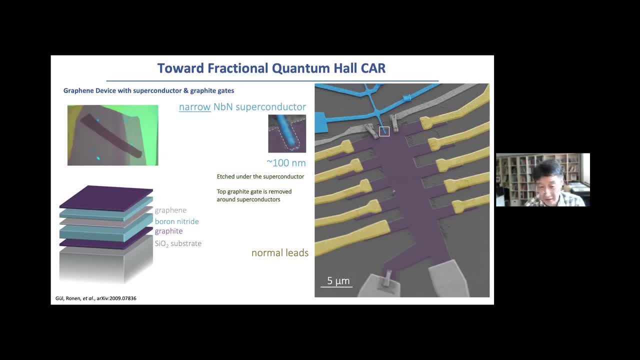 which actually plays an important role. in the last topic I want to kind of touch upon, We made kind of say, many devices and we measure about five devices and that more like the result is the agrees. There are some statistical variations, Of course. we adjust the. 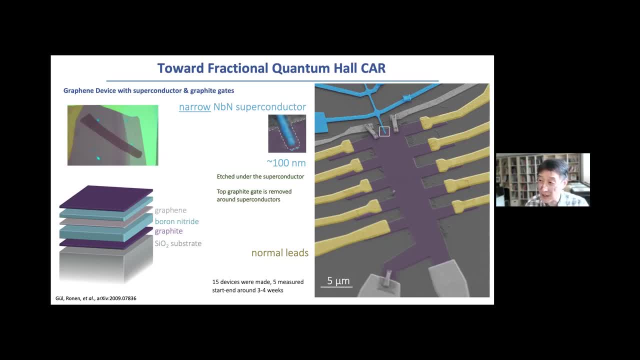 situation. We measure the density of the graphite to the density of the graphite. We measure the density of the graphite to the density of the graphite. We measure the density of the graphite to the density of the graphite, showing the best data But more like the stories agrees upon the many. 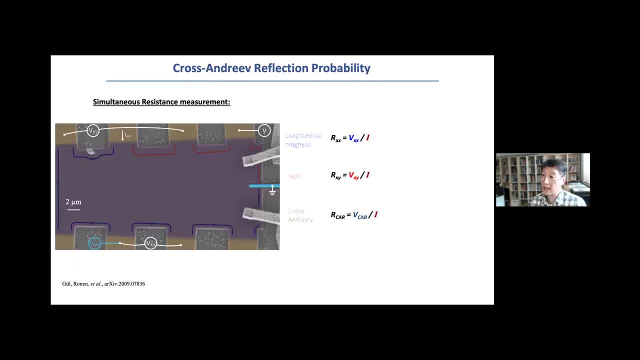 different devices that I'm going to show you. So measurement scheme is following. As I said, we were just inject the current from the upstream, so there's current to kind of bring it down, and superconductor is always grounded and such that the current is always kind. 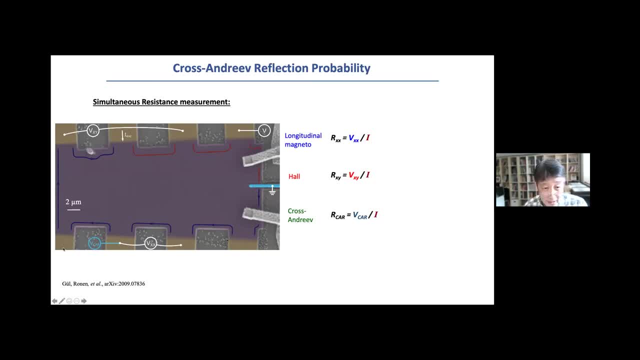 of drained through the superconductor and in the downstream they. basically we can monitor the the chemical potentials to see the downstream chemical potentials. At the same time, we can measure the R-X-X and R-X-Y using this voltage probe and carefully delineate the contact. 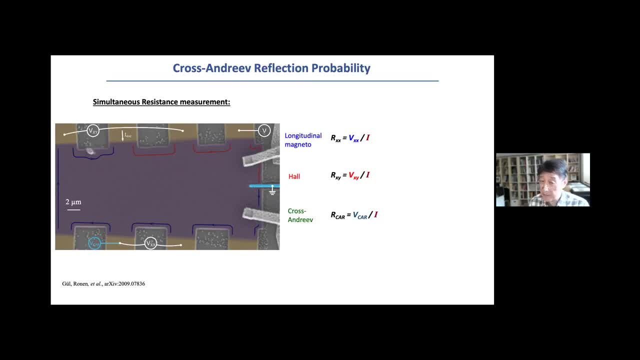 the equilibration problems throughout this. So what do we expect Basically when we measure the quantum Hall effect with the superconductor as a drain contact? basically, quantum Hall effect should not be affected, R-X-X, whatever contact you are making. 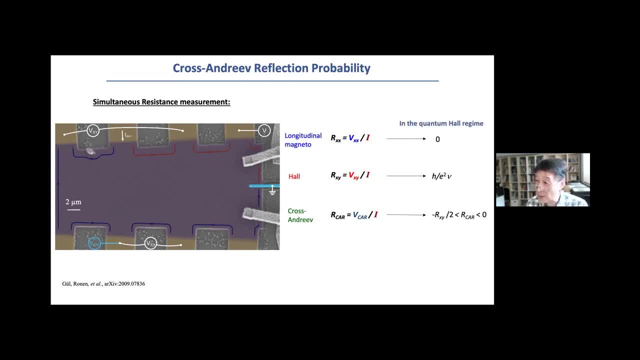 is always quantized, goes to zero. right R-X-Y should be always quantized because it's topological property of the quantum Hall channels. right Interesting part is this: cross-handle reflections downstream. the chemical potentials normalized by the current is arranged between: 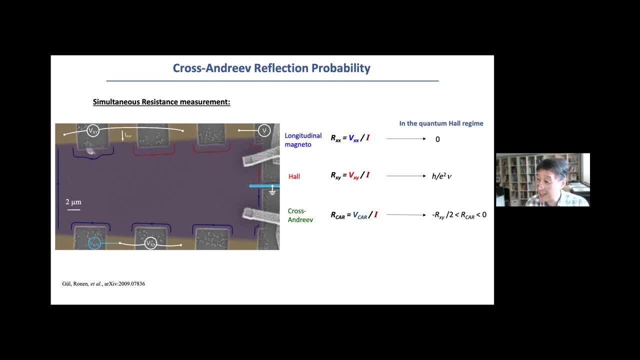 if the cross-handle reflection is happening, it should be negative. There is no cross-handle reflection, it should be zero because basically you are seeing that the carriers coming from the ground and in normal carrier basically expected to zero. So it can be zero to some negative number. 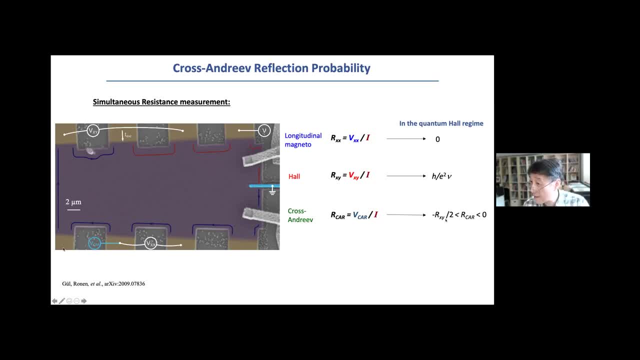 It is bound by half of the R-X-Y if this everything is completely cross-handle reflected. So we know that that's a range of this R-Curve and we can see that strengths of the cross-handle reflections by simply measuring this R-Curve, right? 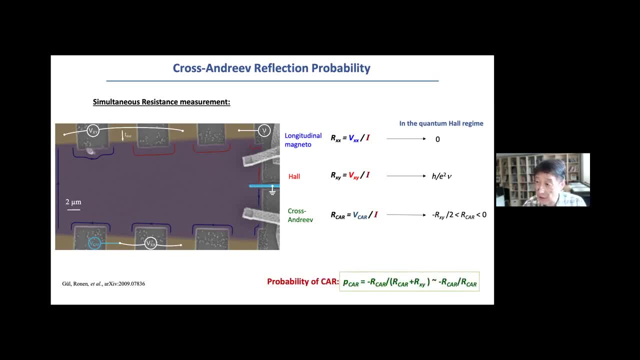 In fact you can just work it out on a bit of math and then you can convert that, this R-Curve, into the probability of the cross-handle reflection per channel. So that's what we call the P-Curve, which is basically obtained for, divided by R-Curve. 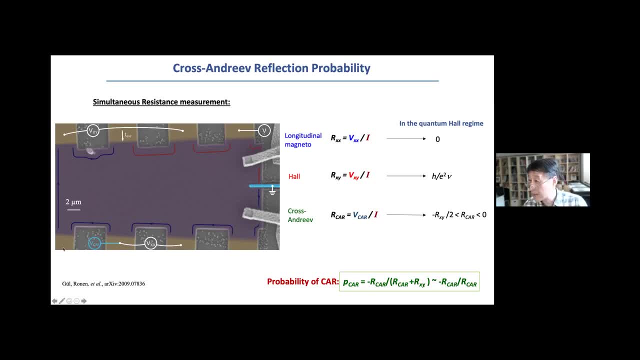 divided by R-Curve plus R-X-Y, But typically, as I already briefly mentioned, R-Curve supposed to be as big as R-X-Y divided by two, but typically this is a much smaller value, So R-Curve is smaller than R-X-Y. 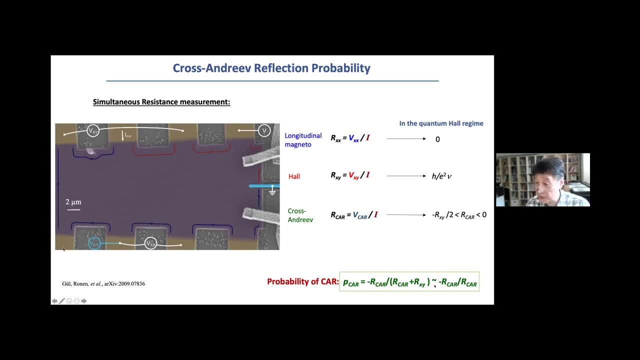 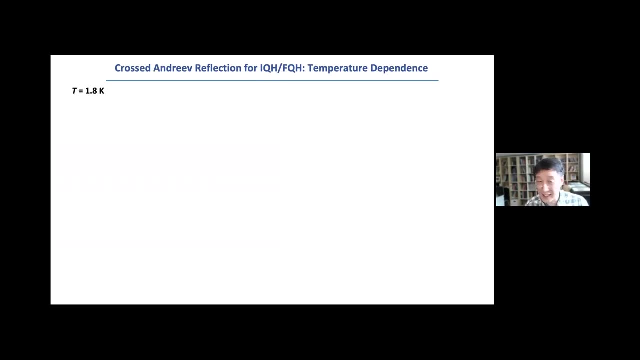 which means that usually the probability of the cross-handle reflection is obtained by taking the R-Curve divided by R-X-Y of? sorry, what is R-Curve? R-Curve divided by R-X-Y? So there's a typo here. So that's kind of the how you want, kind of look at the data. 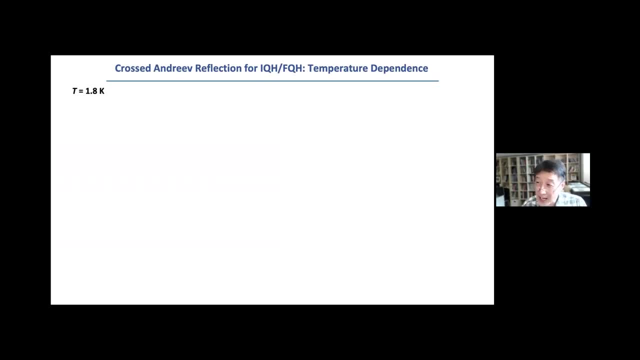 So let's look at the data now. We did this much higher quality sample than what we made four years ago. We can do the following experiment Already, at 1.8 Kelvin with a magnetic field up to the 14 Tesla. clearly that this R-Curve. 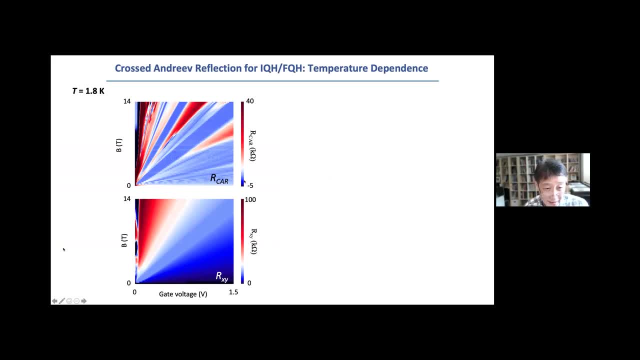 I'm showing the R-Curve in terms of the color negative signal is something that bluish. you can see that. okay, R-X-Y showing that this the typical band, like the behavior that you're seeing, that all this quantum hole band diagram. 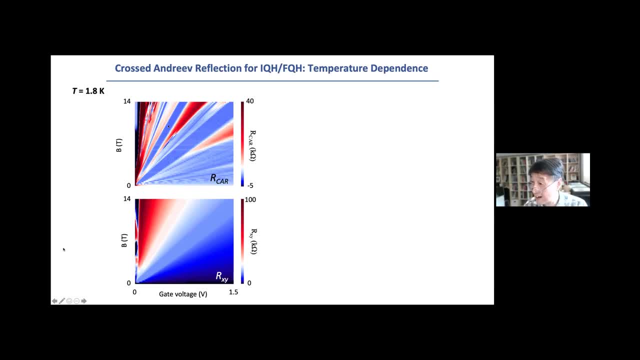 but our car shows that many blue stripes, which means that the car process is quite strong. but more exciting part is that, rather than integers, you see that a lot of the fraction car process already started to show up, So this is very encouraging. 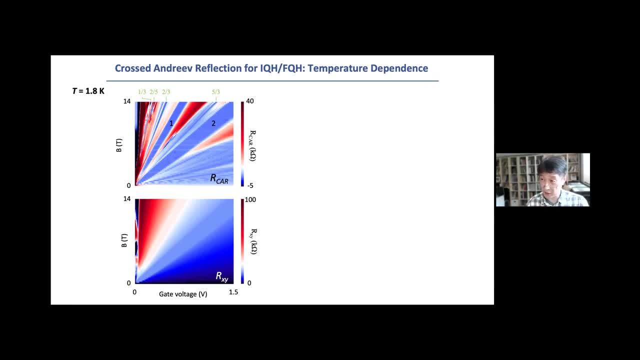 With this device. already we see that many of this fraction quantum effect do appears as a negative cost. signals into the signal, A little bit of cross sections at the high magnetic field. 14 Tesla. you see that the R-X-Y shows nice plot. 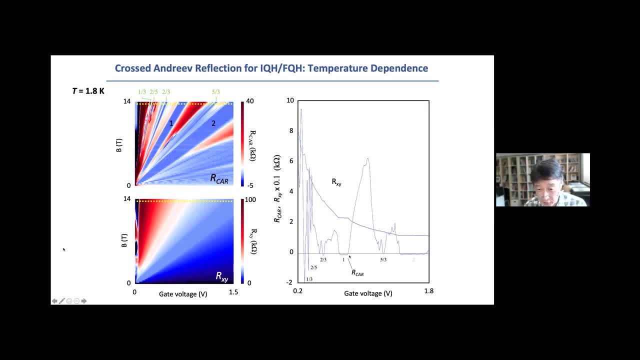 of response to this, all the quantum hole sequences, including one and two, but, more importantly this, fractions and fractions, And, as I just mentioned here, shows a large negative car process value. So which, actually indicating that indeed a car is very robust into the fractional quantum hole states. 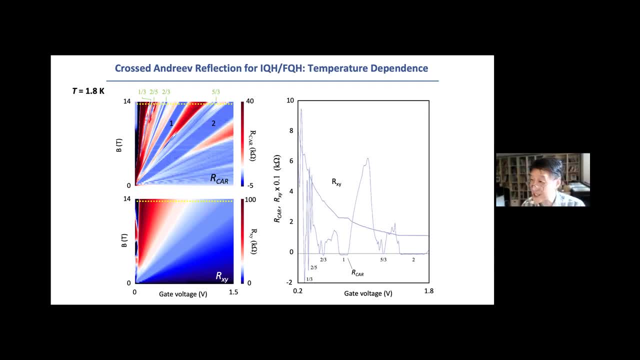 Now to make sure that often that this type of the experiments will just bring it up experimentalist and even theorists to ask that are you sure that this negative is not an experimental artifact? So one thing that we can just do, that is: it's the same. 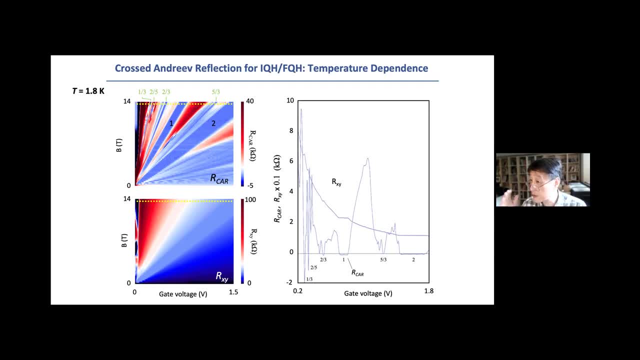 management. we simply increase the temperature, especially go beyond the superconducting transition temperature right And superconducting becomes a normal contact. And then how this car signal process? I think that is one of the important criteria we should kind of show. 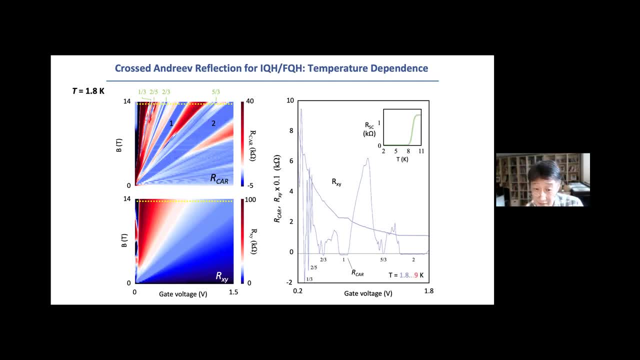 indeed this nitrogen nitride tc is around right A Kelvin. when you heat up the system beyond A Kelvin all the negative signal is completely go away and completely turn into positive. And it becomes positive because the car process, car measurement, is kind of three-terminal measurement. 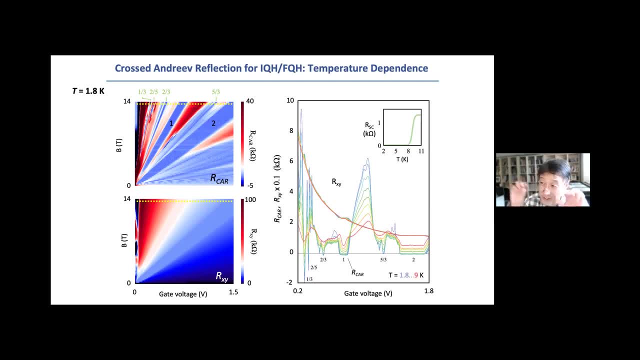 So inherently include some part, especially the part of this contact resistance, And that's kind of naturally expected. But this actually show that indeed, car signal, we imagine, is rather the intrinsic effect. we are seeing that related with the superconductivity right. So before I just hit back, 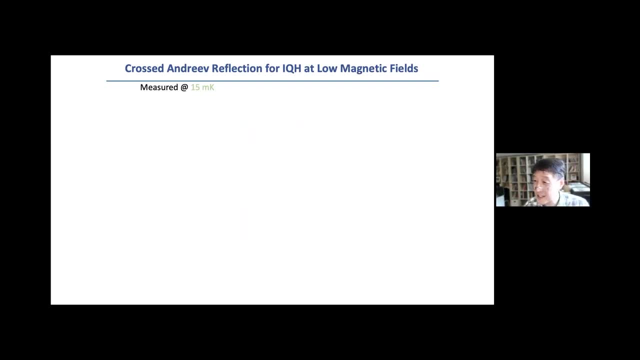 to the fractional quantum mode effect. let me just kind of briefly discuss about the integer quantum mode effect already, which are also already quite interesting. So let's say that if you parked around the full Tesla- not full, no full- the fractional quantum mode effect fully developed. 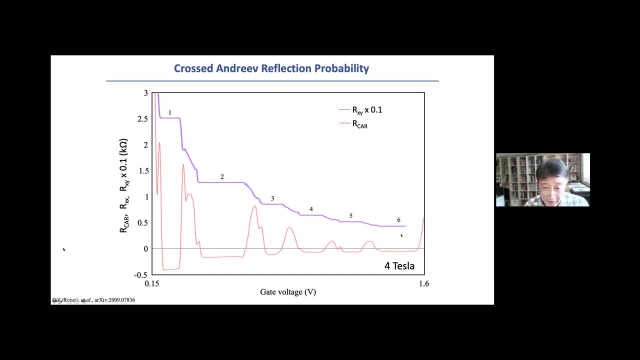 we already see that the one, two, three, four, five and those kind of the Rxy shows up here At the same time. car actually shows up very robustly in the negative values right: One, two, three, four. 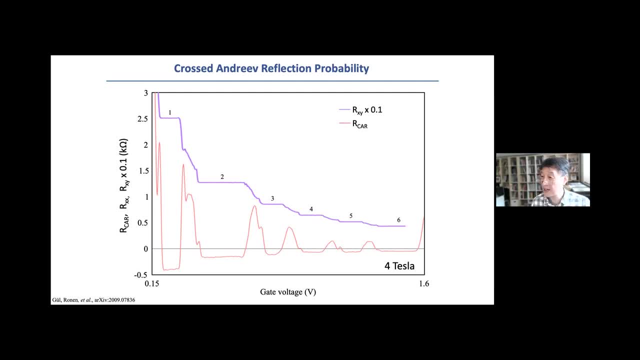 And you see that whenever there's quantum or plateau appears, then you get the negative R car value And you see that car actually increases as you go to the lower filling fractions And we scratched our head why actually it's increasing. But we found this interesting. 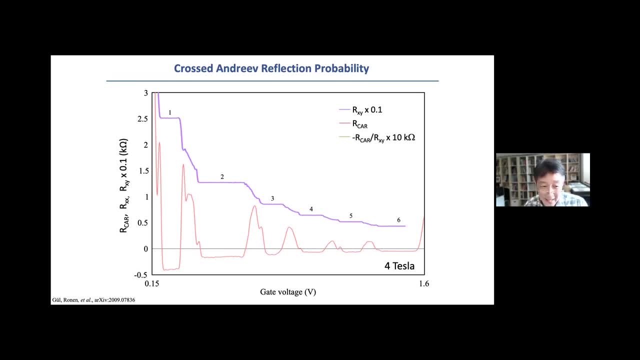 that if I just normalize our car with Rxy, basically they are more, more like the same values. right At this point you start to remember that, indeed, that I mentioned that probability of the car per the quantum mode channel is proportional to the R car divided by Rxy. 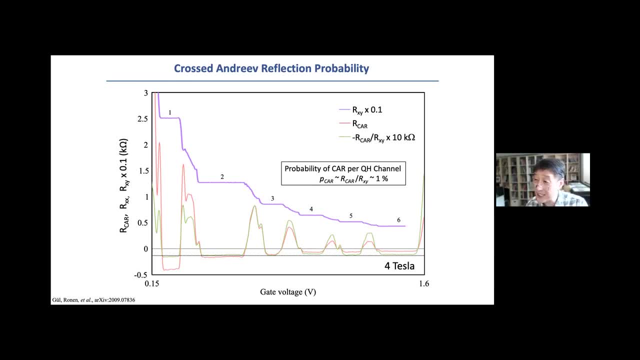 This means that, regardless of this, how many edge state I'm impinging onto, the system per states, per edge state car process is exactly the same. You equal one, two, three, four, right, And this actually is a very robust. 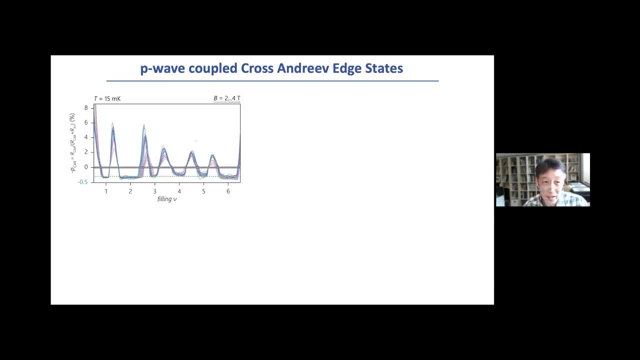 We just measured many different integer quantum mode effects between just magnitude two to four Tesla. As long as this quantum mode states sets in in all integers, including the so-called the symmetry broken quantum mode edge states, as long as integers we get basically very robustly. 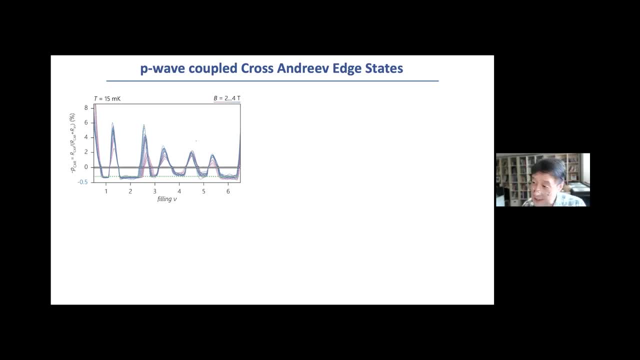 that all this car probability is the same. I think this is rather intriguing. Why is that? Because some of the edge state is a far away from the superconductor, So naively we expect to see that that that will make the superconductor. 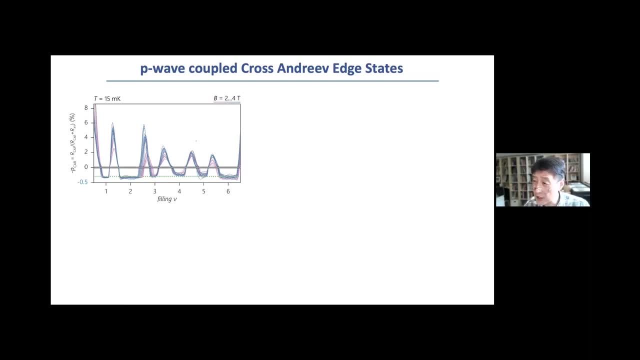 that will make the superconductor, that will make the superconductor, that will make the superconductivity, the proximity effect, weaker, but nevertheless, top probability is the same And it turns out that this is basically expected. in a sense, it actually support. 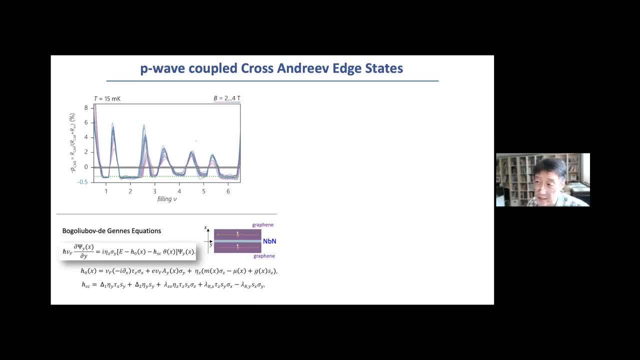 indirect support of the topological superconductivity we are creating in the system. So, theoretically, if you just try to understand this one, basically you just solve this. BDG equations, including the superconducting, superconducting, thin wire, the two quantum or edge states. 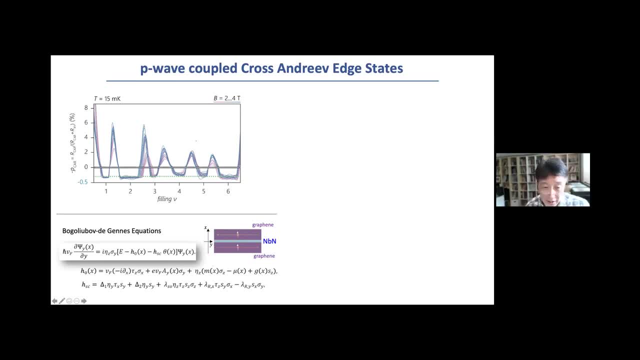 the up and down, the count, propagating the opposite directions and running down in the system and use it, basically approximately ties that this two quantum or edges right, It turns out. it is a very important that we have to include, especially when new, equal one type of things. 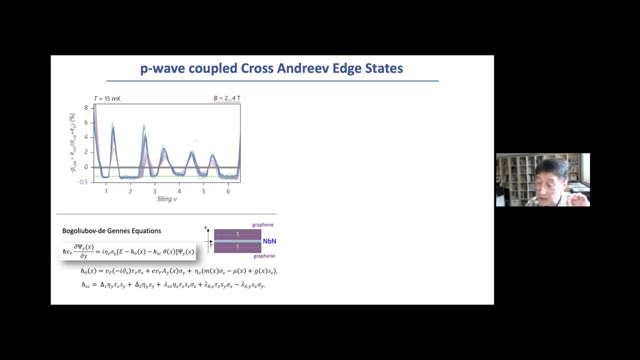 quantum or edge state where spin is polarized. including that the spin of the coupling inside of superconductor is a very important because naivium is a heavy metal And we expect to see that. expected have that there's a reasonably strong spin of the coupling. 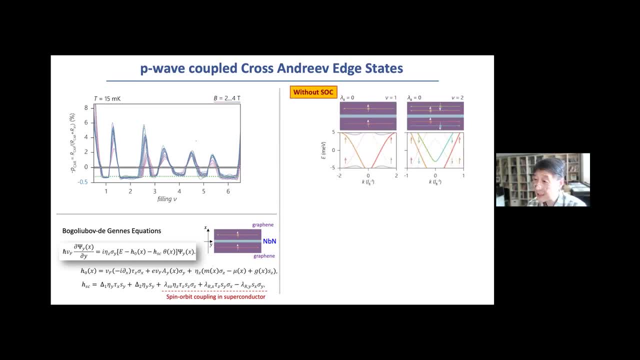 And that is very important because without that there is no way that I can make the decoupling between the two spin polarized edges state in the new equal one right. Basically, I need kind of from the single pairing therefore the I have to really remove the spin indices. 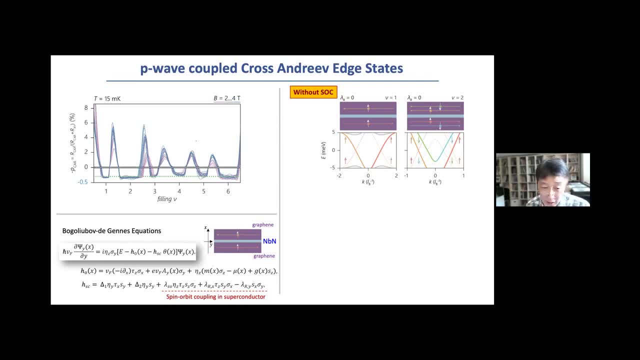 or make the spin is not a good quantum number anymore, by just including this spin of the coupling. Now, if you just include this regional strengths of the spin of the coupling, it turns out that the spin of the coupling, it turns out that then it opens up the 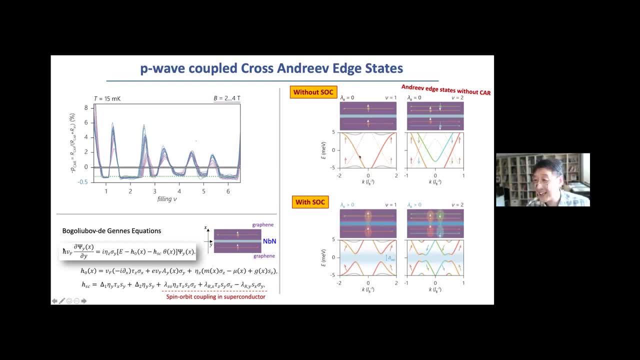 this, the two independent the states basically couple each other and open up the gap. And this induced gap is kind of directly related with the size of the spin of the coupling. So that's as well as the superconductor, So that is kind of interesting part. 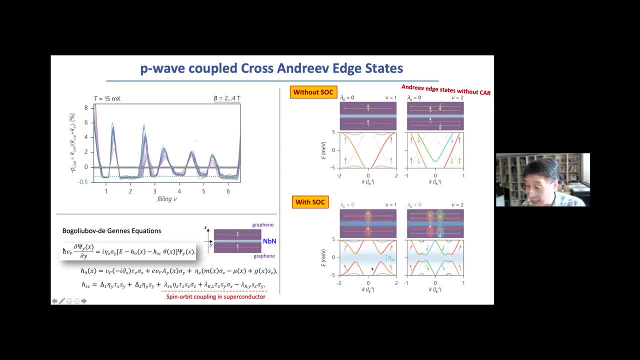 And important part is it opens up the gap- And this is basically a topological gap in a sense- that ensure that there's a zero mode Inside of the, in the mode which actually mediate this kind of the cross under process. 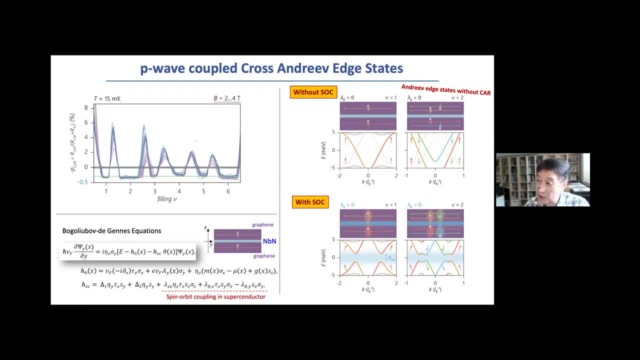 Because of that, in a sense, that every time I just add up the quantum edge state, basically I'm adding up another copies of this type of the topological gaps, with the zero mode in there. In this simple view, therefore, that regardless of the details, 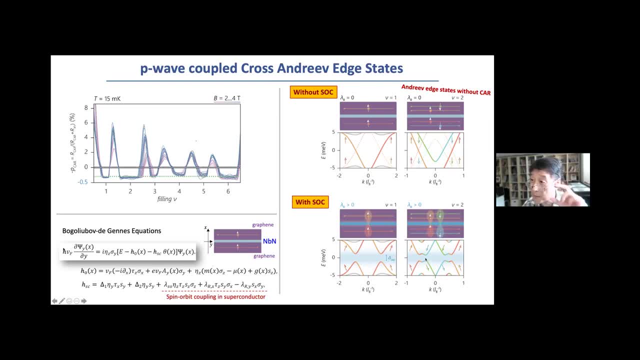 of the size of the gap opening. basically, as soon as the gap opens up and it's resolvable, I expect to see the basically very similar car process. This is happening And that is what we are seeing: the experimentally very robust car probability across the system. 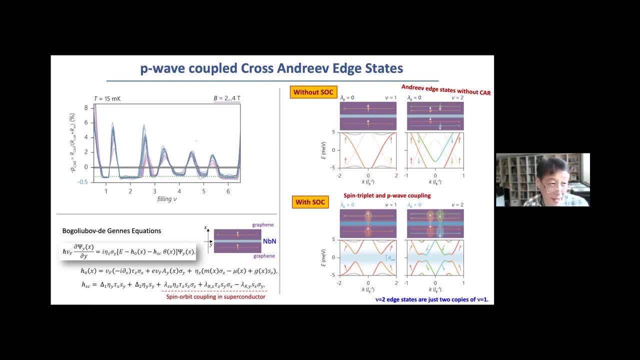 Why the car probability is so small, about a few percent, about a percent or 0.5% in particular case. It turns out as soon as you just can include some of the barrier, like the pump, especially in this particular case, 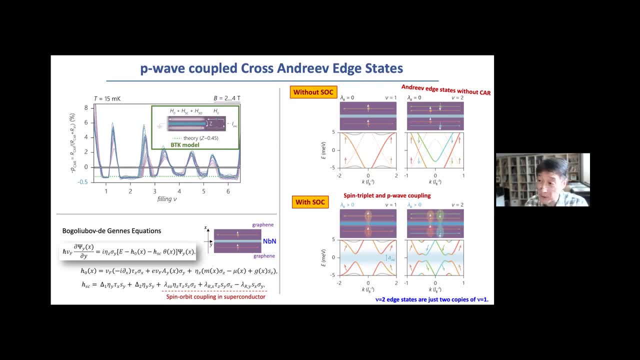 core tunneling of the carrier is spoil this process. You quickly start to reduce this car probability And typically the Z number we just include there is something like about 0.5-ish. then you get the about kind of few percent of the cross-country process which is happening there. 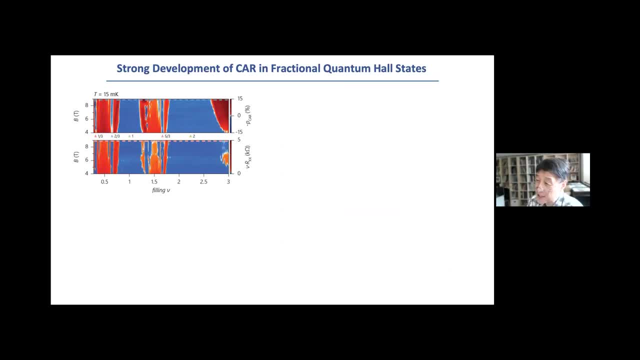 Right Now, with this, let's kind of move on to discuss about what is happening in the fractions. In the fraction, basically, as I said, there's a robust fraction is happening In fact. the fractional car- Yes, Yeah. 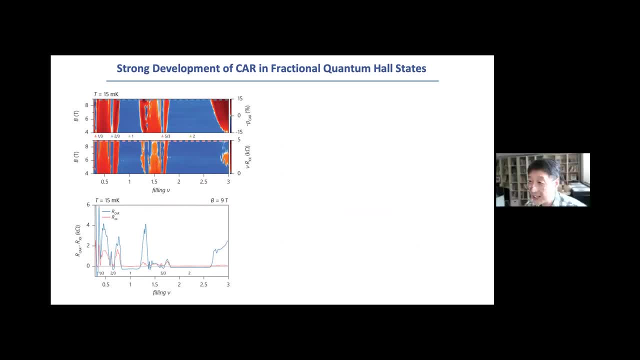 How many minutes more do you need to wrap up in? about five minutes, I think All right. Five minutes is probably enough, I guess. Hopefully, All right. sorry for the interruption. Yeah, so that's okay, I think yeah. 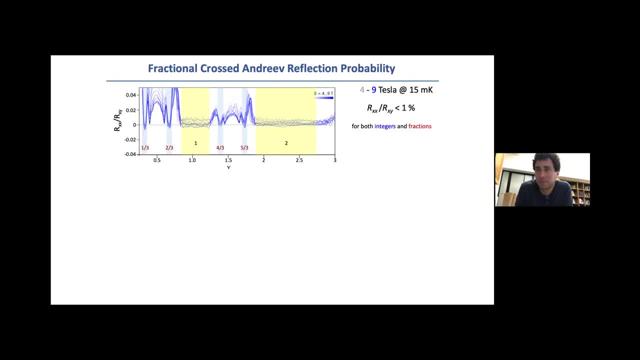 So let's see that, let's hit this nutshell. So, basically, fractional quantum artifact, the car is even stronger, right? And even if we just kind of cross the convert into the P car, that it's generally stronger than what is a P car. 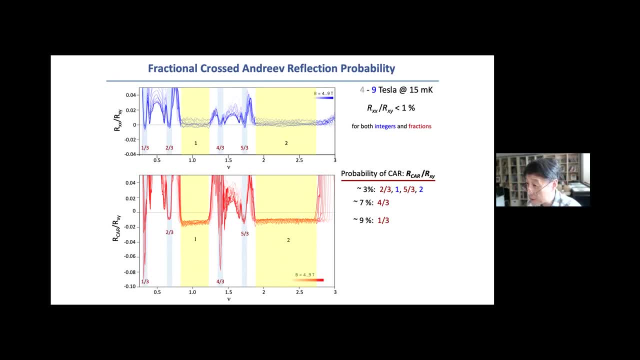 the probability that you get in the integers. So it is a very robust. and it is even more robust when you get into the sum of this fraction, especially fractions less than half. so include one third and two fifth, that there is tendency that a fractional car 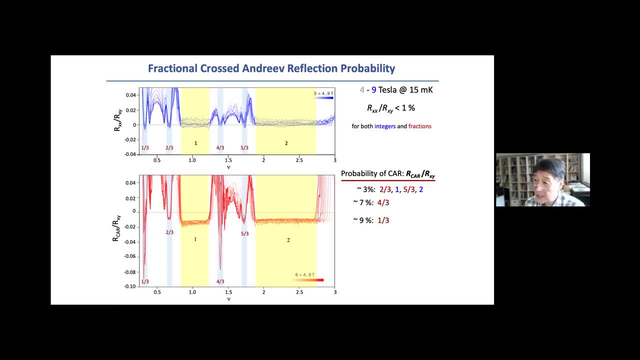 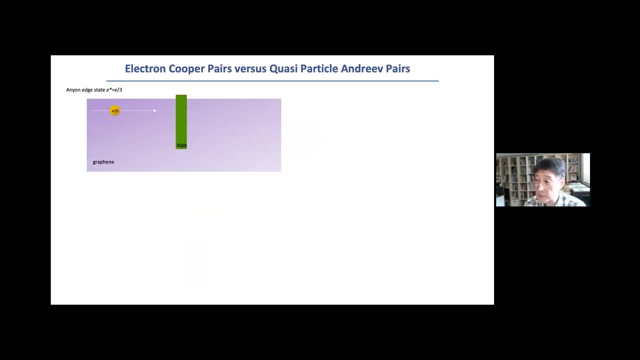 is even stronger than what is seen in the integer. So it actually brings us to kind of some of the wonder why the fractional car process is even stronger, and especially stronger at the lower temperature, And there's this kind of some of the scenario that we can think about. 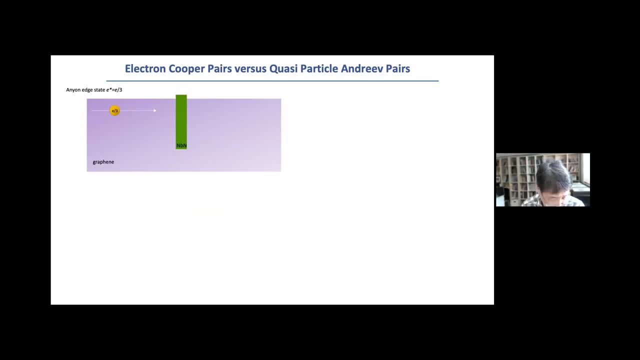 What actually makes this a process, the fractional car, One way that nine way we can think about is basically: I have the edge state of the fractional quantum artifact that comes in with the say: one third state, one third of electron charges. 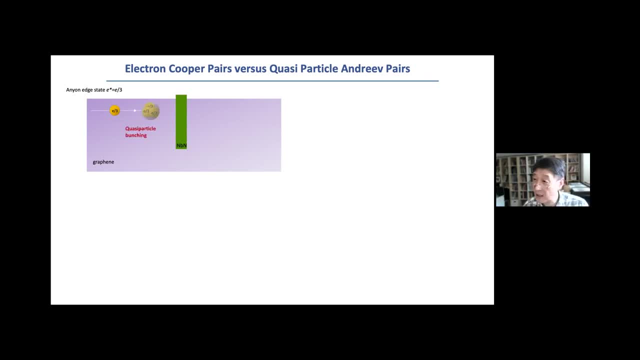 The way that I can just kind of put this car process is: I will just collect all this one third charges to make the one charges right And then I can form this basically a regular cross-undue process to form the group. 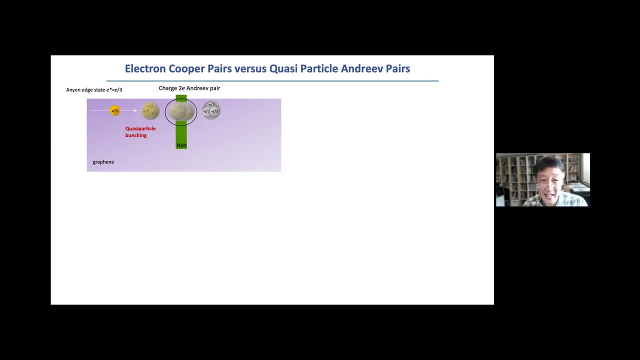 or pairs, and then charge two Yandere pairs, sorry, and then make this a hole in the other side and this hole will, downstream, should break down again to the one third of the whole charges, And that's kind of one way we can think about. 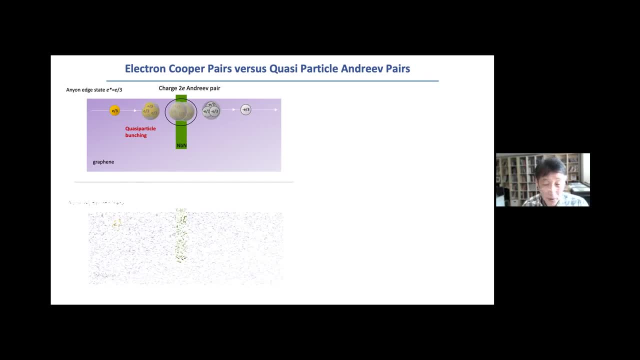 to making this process. The other, more thrusting idea is, instead of that, bunching this one third charges to make the full charges, to make this 2E-Yandere process. maybe you can conceivably think about getting this 2E state. 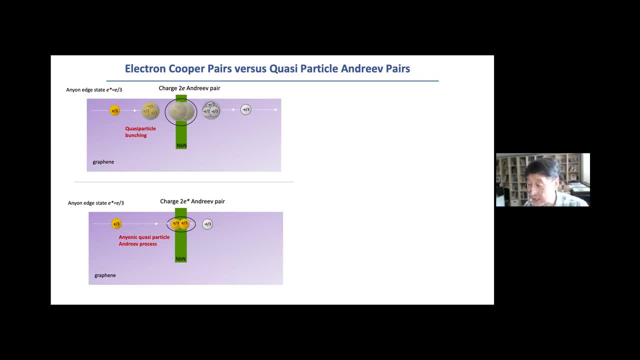 the star of this Yandere pair or any Yandere pairs to make the process can happen. In this particular case, I don't necessarily need the bunching. In fact, the theoretical argument tells us that in the upper cases the charge 2E-Yandere pairs. 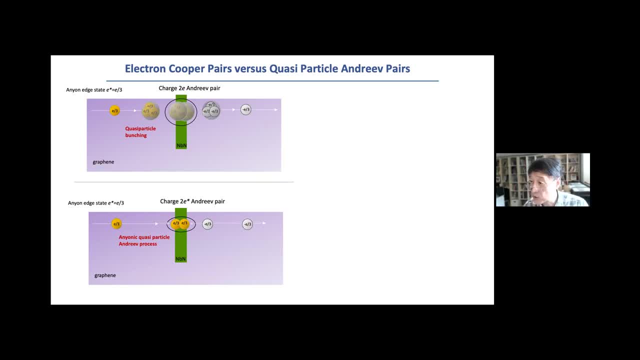 since you need a bunching process. it actually costs the energies, which means that as you go to the lower temperature it tend to be suppressed, while that this the charge 2E star of the Yandere process, this- there is. no bunching is needed. 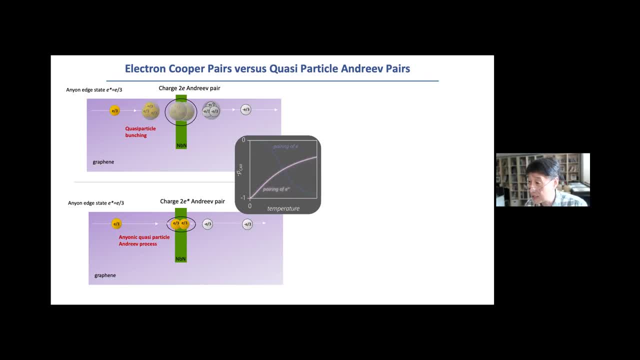 If this is indeed the ground state, kind of close the ground state properties, In fact, you expect to see that a stronger the process happening at the lower temperature. So, temperature dependence, they actually tells us that these are distinctions. Indeed, when we just look at the temperature dependence, 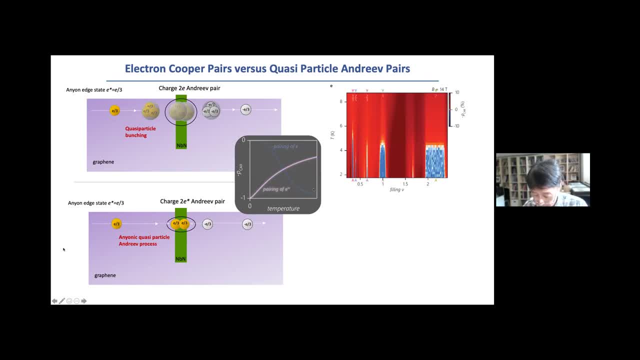 of the car process, with the temperatures, with the car, we found that indeed this the process for especially one third and the fractions, and that two fifths is stronger as you go to the lower temperature. strongly support but the idea of this charge. 2E-Yandere process. 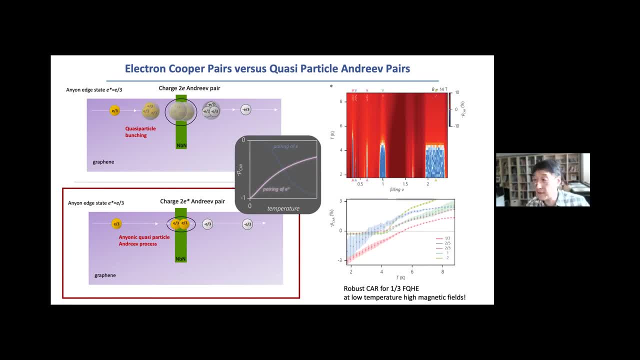 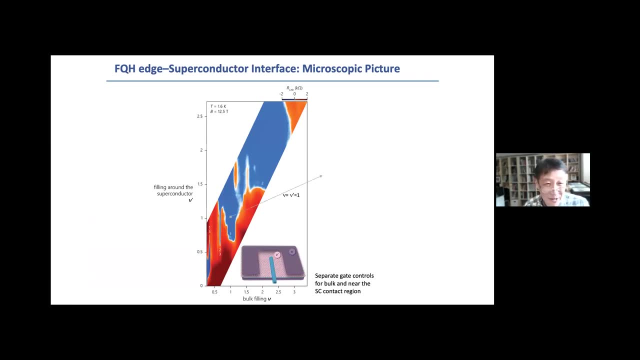 in other words, it indirectly proved that the existence of parapheromone states in this type of the system. I know that Jerry is kind of now pushing me, So let me not go into the details, but all of these things also can be carefully discussed. 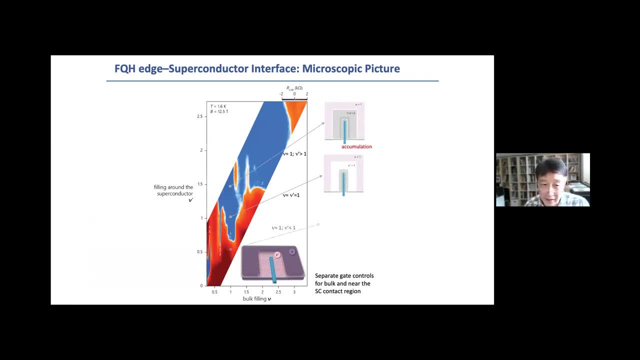 again by changing the chemical potential near this contact area And just kind of we can just take a look. Indeed, one third and the two fifths actually goes to a rather different process with all other integers or even all other fractions in the higher filling fractions. 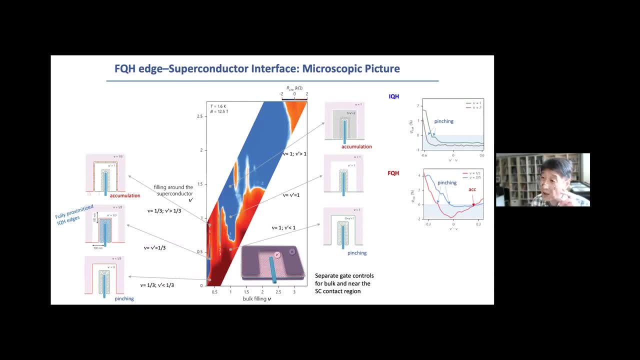 Also strongly indicating that, indeed, we are seeing the fractional car processes rather different from this integer car process, And that's basically indirectly support the idea of the formation of the parapheromone, in my opinion. Okay, so where are we going? 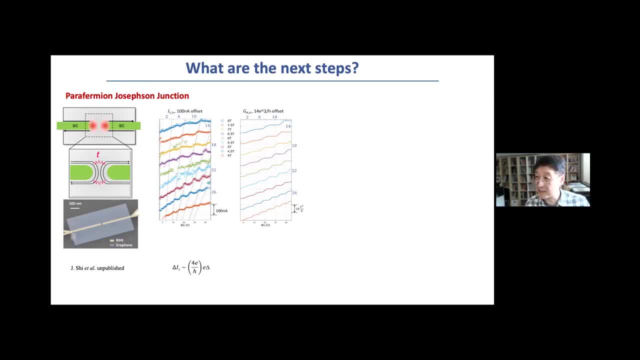 So we have to really just show the next step, Indeed the existence of parapheromone. There are many different ways We're graphing. One can also make this at the Josephson junction. Already some of the efforts we are just providing. 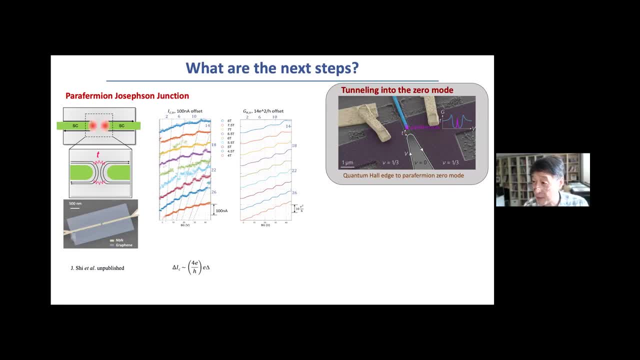 or we can just follow through the semi-conductor wire type of experiment, We can try to the tunneling experiment, the end of the superconducting wires where the parapheromone sits in, or we can try to even just directly measure. 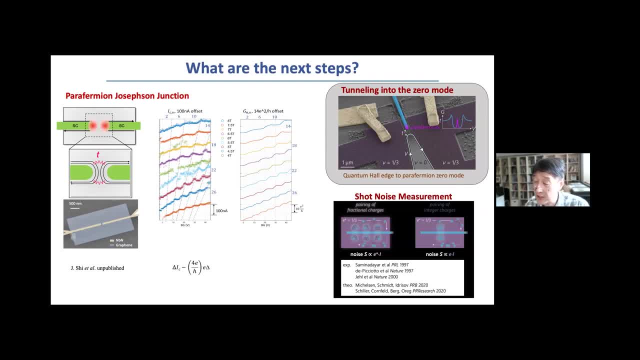 this fractional car process, basically measuring the short noise type of the measurement. So that's kind of something that we are thinking about. Thank you, Thank you, Thank you. Very nice, I would open it up for questions. I just wanted to express a wish to actually 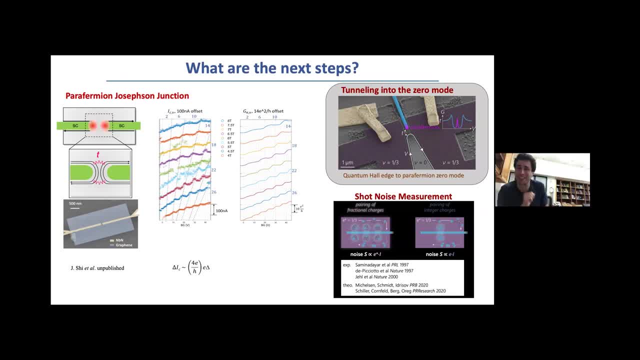 yes, ask you a question about the parapheromone cause and error reflection, So maybe I'll start out by asking it. So you were suggesting that there's a possibility of one third coming from the left, and was it minus one third coming from the right? 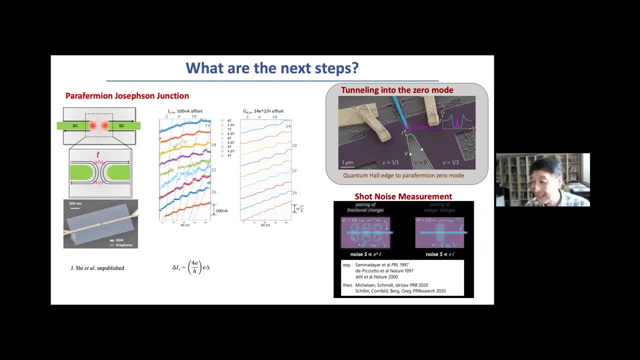 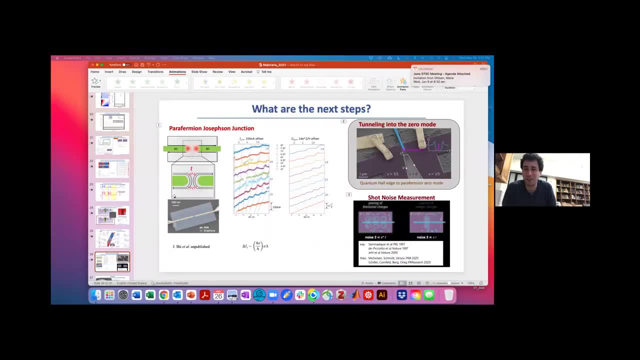 Is that right? Is that right? Is that right, Yeah, Yeah, Or is that right So that that will give you definitely a little confusing. So let me try to clarify. So the constant drive reflection electron comes from the left. 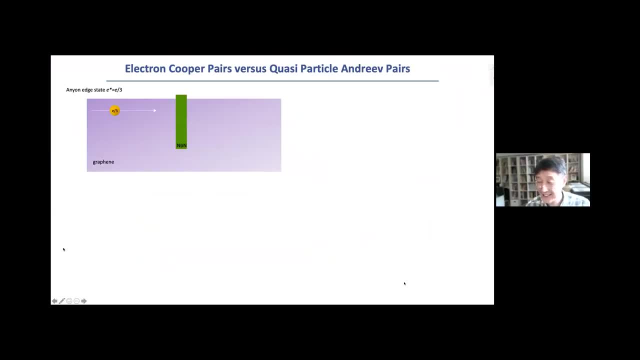 electron comes from the right comes out as a Cooper pair, Yes, But here it's right. Let me see whether I can do it right, Right, Whatever things. let me just see that. I think I have even better. I think, yeah, no problem. 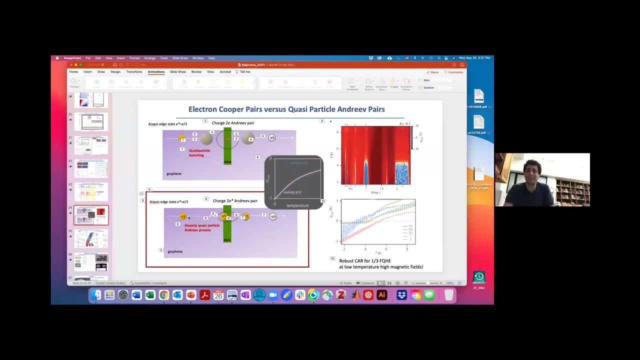 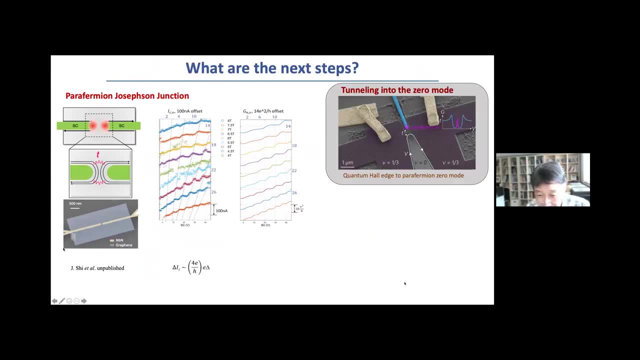 I think let me see that one. Okay, Yes, yeah, exactly, Guys are a bit better diagram, So let me just show you rather than so, let's see that you can see here, right, So the process that we are proposing is indeed. 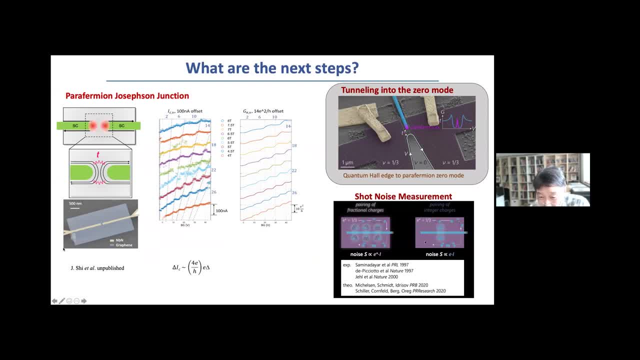 indeed, this is a likely than this one right. So the we have the one third coming down here in the downstream. basically it's one third of the whole right, Yep. And then we form this: the one third charges of the undrive process. 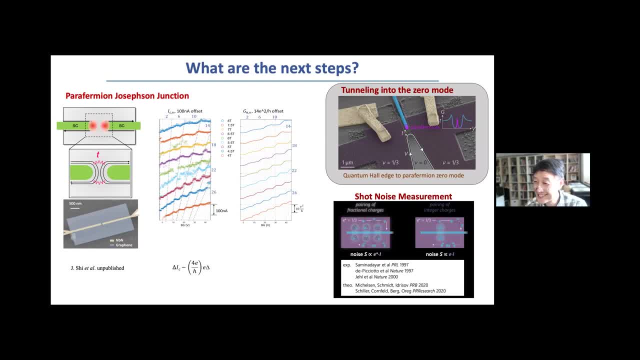 Basically that is the proposal, But then and then you have like a two thirds E coming out as a Laughlin-Cooper pair. Not sure whether I can call this a two third of Laughlin-Cooper pairs. I want to say that this is basically a undrive. 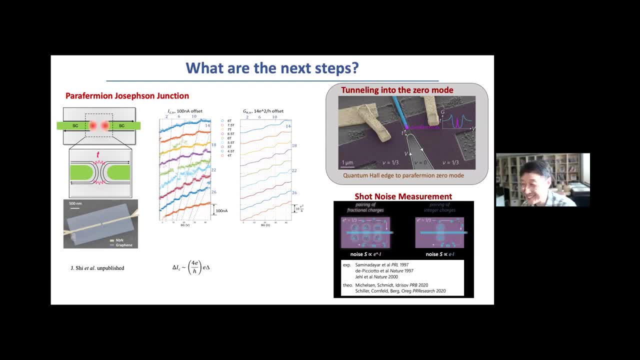 pair of states of the one third charge. That's a kind of yeah Well, I think maybe it's something that you can. you can just put it in a different way- right, Yeah, But you could also have the one third coming from one side. 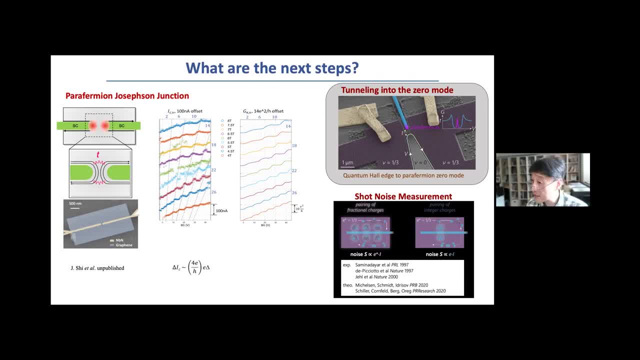 and five thirds coming from the other side. I think that's. that's in principle. that's also kind of possible. I think there is no restrictions, except that in the end of the day I'm having the far away superconductor. 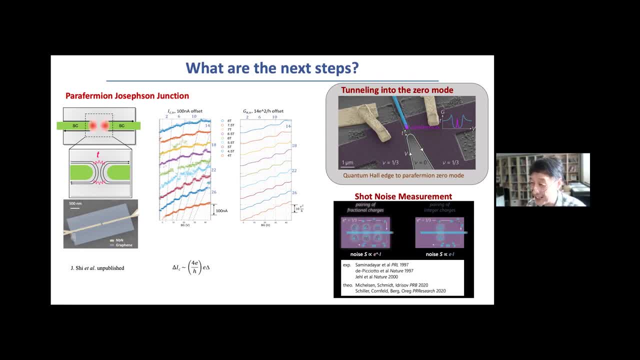 Anyway, I should see that this is just the one third of the charges. the quantum, The more edges right. So not sure whether I can just change even that, especially far away from the superconductor. So I don't know whether I have the other choices. 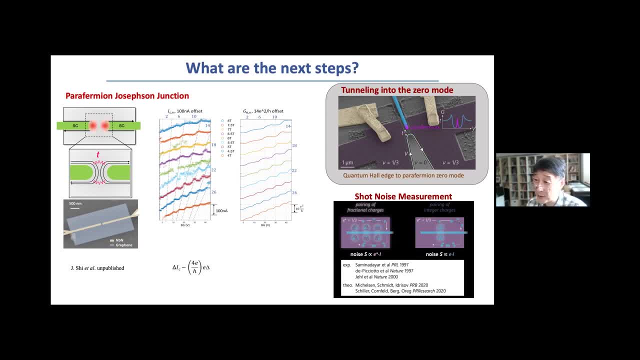 than this one. but this is a kind of good good point, I think at this point this is just a naive proposal, right? And then the experimental evidence I can present here is only the temperature dependence of the car process other than or other. this 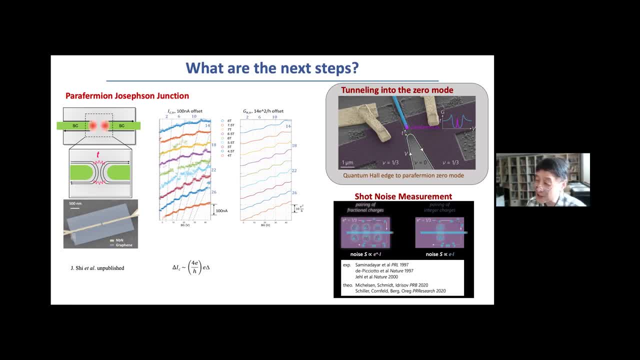 the outlook type of experiments. So any of the things that I just draw cartoon, you have to just take it. There's a grain of the sort: This is cool, Brings back good memories from the theory work. Anyway, let's take one more question before continuing. 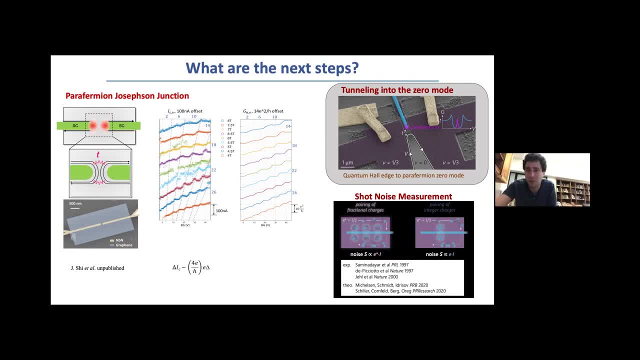 or let's see. So maybe two more. So I see a question from Kirill Shnichko. Go ahead. Hi, I wanted to ask this question. You talked a bit about the spin orbit coupling that you need to make for the two edges. talk to each other. 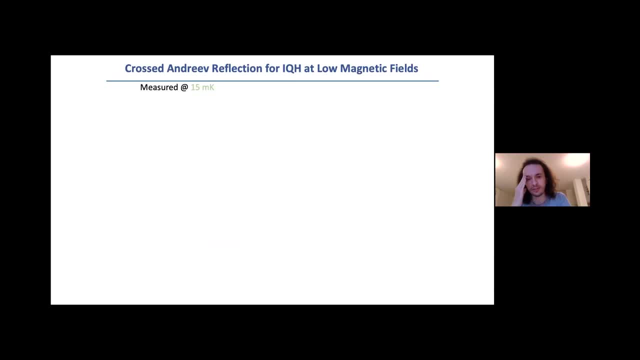 And in Moti-Heibloom's group there is this strategy to make two quantum wells and gallium arsenide and bring two edges of opposite spins close to each other. I wonder whether this is possible with two layers of graphene, And I have a suspicion that even by layer graphene. 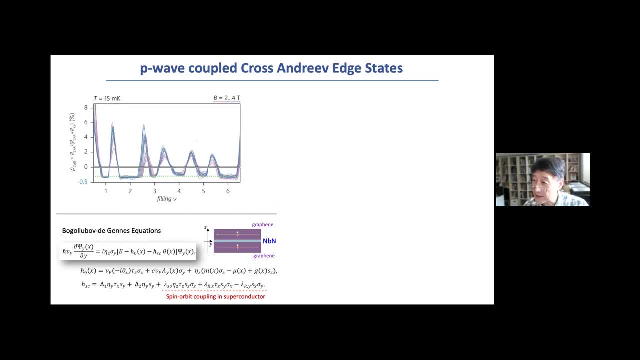 would work for that purpose. Yeah, that's right. Good point. I think the original theory proposal is indeed that comes with. I think Jason's proposals comes with the in fact to put the gate on the half and just kind of try to convert into the opposite side. 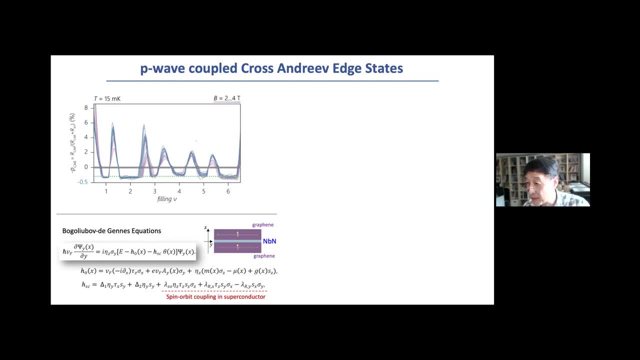 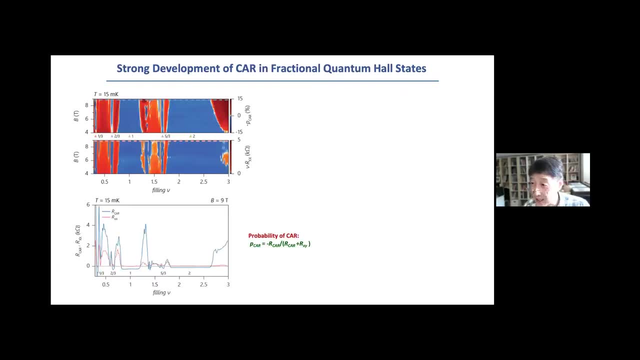 such that you don't have to bring this spin or recoupling arguments, but basically you flip the spins on the other side. But as you just kind of rightly mentioned graphene, those kind of geometry can be done rather than putting this lateral gate. I think that is one. 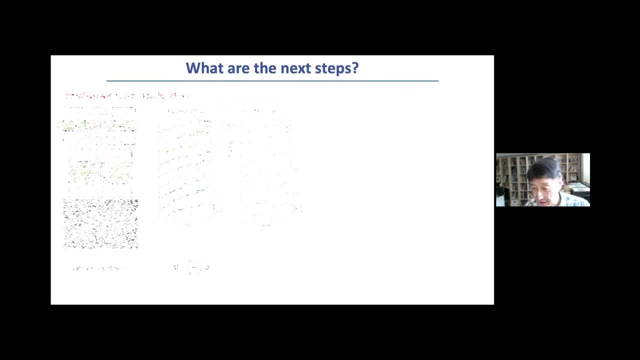 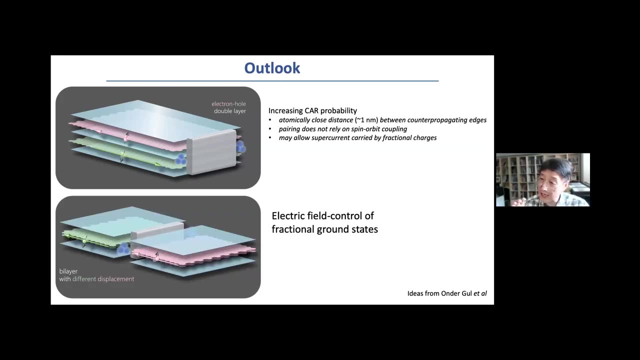 Yeah, here we go. Yeah, something like this is what you're saying, right? So, indeed, the kind of- we are just trying to get this not onto the trench type of the geometries, but you can also put the double layers. 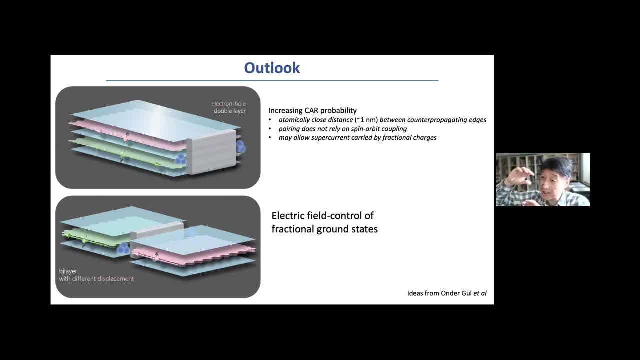 And if you just the gate in top and bottom layer, and then you can make this whole lambda level and electron lambda level and the spin is opposite directions, right, And then still you have the nu equal one, for example, or the fractions, and then you don't have to rely on the spin. 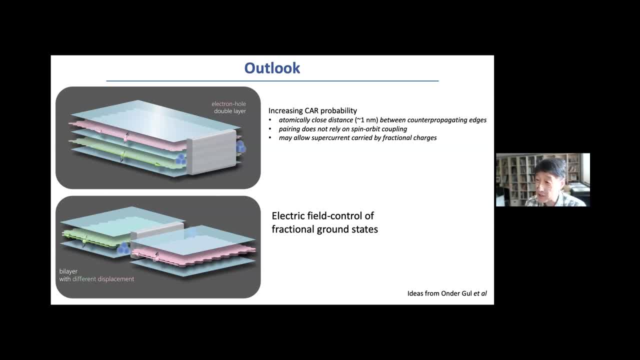 or recoupling anymore. I think this is kind of interesting idea. We are just trying to also pushing this experimental side. We don't have yet the convincing data, but certainly that is one of the conceivable experimental idea we can implement. I see, I'm excited to see the results. 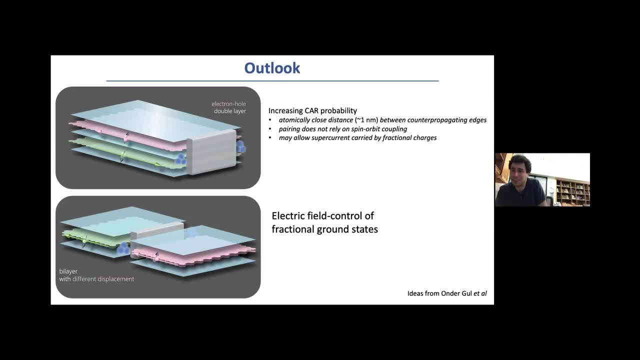 Let's go on with a few quick questions. Alexander Stasiowski, You are muted. Alexander, Yeah, Oh, thank you. So I wanted to ask you, if I remember correctly, is this old suggestion or proposals of Shushan Janketal? 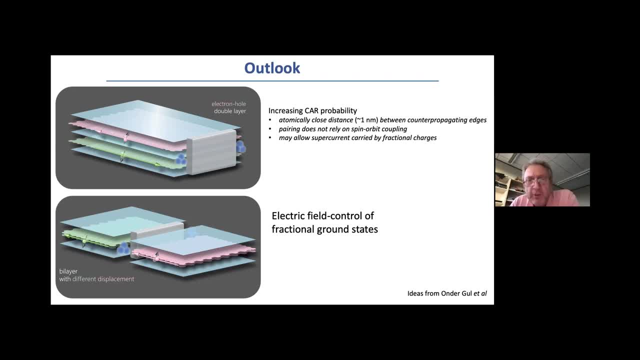 when you put a superconductor on top of integer holes. let me just see myself integer hole. So there was always this picture in which the edge mode, which is Dirac mode, would split into two Majorana edge modes and one would go around. 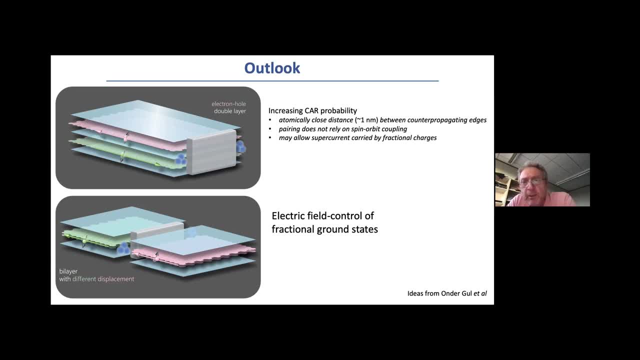 and one would go just where original edge was. And in your case it looks like there is nothing going beneath the superconductor, so both mode go around. So I just wanted to ask: why is it so? why is it different? Right, I think. let's see the weather. 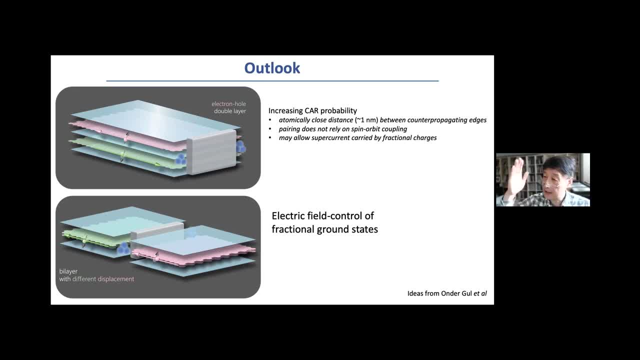 So there are indeed kind of discussions that the edges between the superconductor and the quantum or channel, basically you expect the Shushan Janketal, one of the papers described that this idea, the edge state, can be decomposing into the two Majorana state. 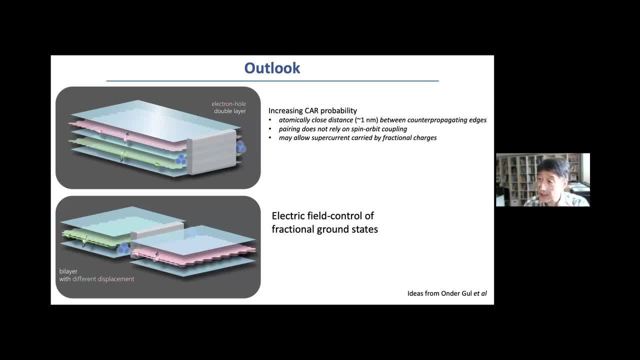 to traveling with a different speed, right. So that's kind of one way. Now I think that can be mapped back. I believe that can be just mapped back into the. in my language is basically this: cross-andrive edge states or the solid andrived edge state electron hole.